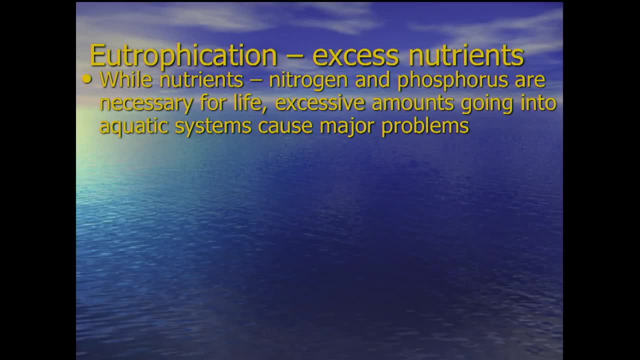 everybody knows you need it. You need nutrients. Nutrients are essential for life and two major nutrients are nitrogen and phosphorus, and we need that in our food. but when too much of it gets into the water it can cause problems In marine and estuarine environments it's. 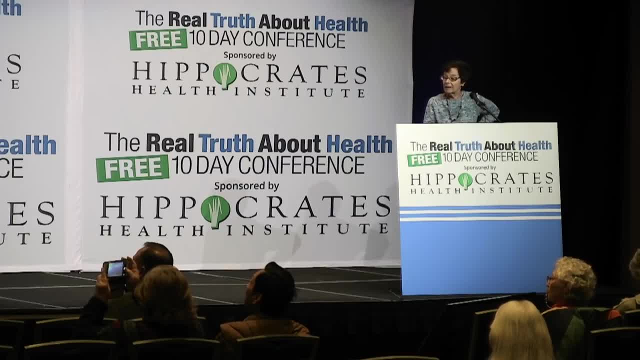 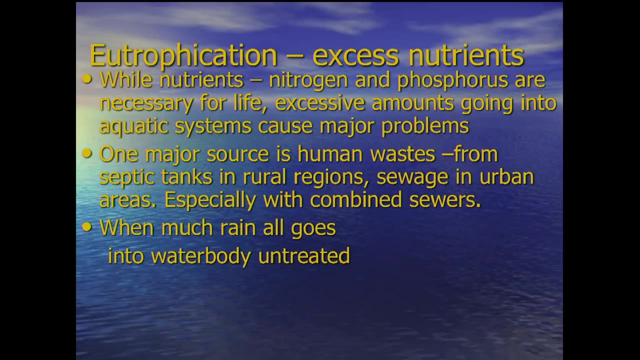 nitrogen is the major problem. The major sources of this include human waste from septic tanks, from sewage treatment, also waste from farms, like fertilizers and manure. When there's too much, it goes into the water and can cause problems In urban areas such as New York City, older cities. 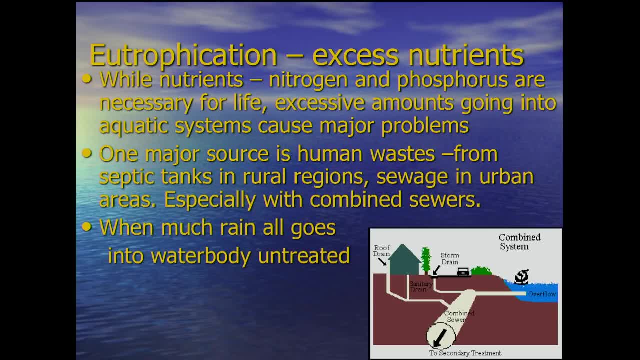 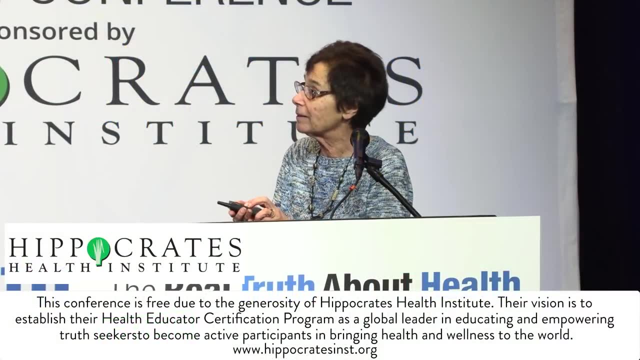 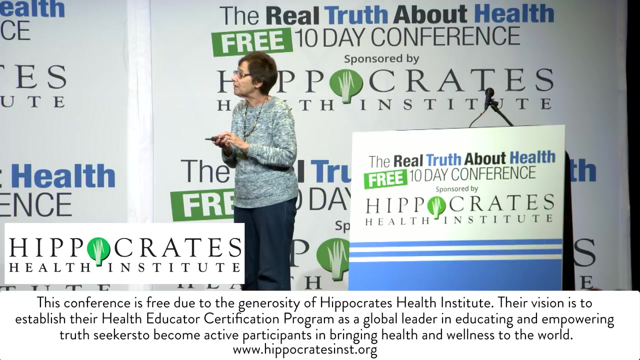 where there are what's called combined sewer systems. What that means is that the sewer system- let me see if I can get a pointer here- The sewage from houses or industries. can you hear me? Okay, Okay. 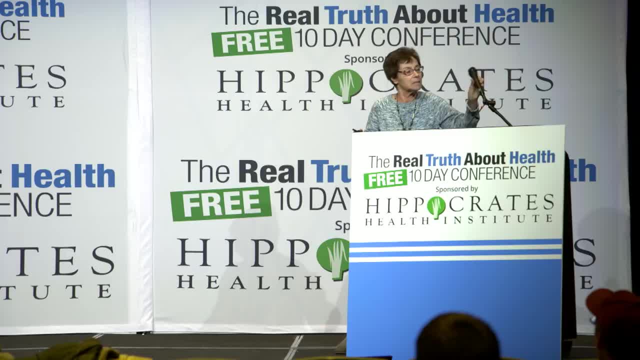 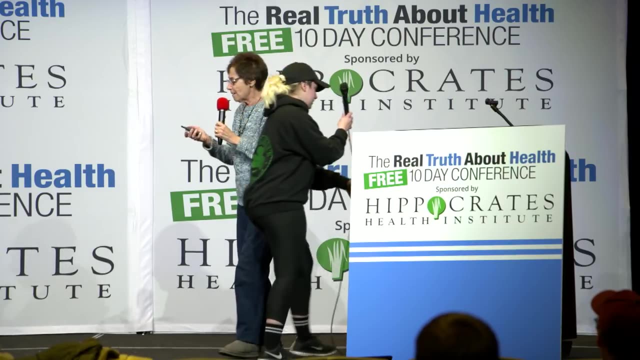 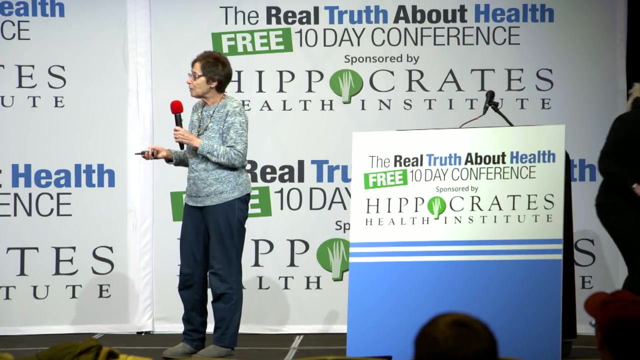 Okay, okay, I think I can take this one with me. this is okay. all right, let's go. let's go here. this: the pollution, the sewage comes here goes down the pipe to a sewage treatment plant. they thought, and it was a really good idea at the time when they built the systems that the wastewater from storms going down storm drains instead of going right out to the water because it would pick up pollutants on the way going down the street. it would pick up horse manure, dog manure, whatever. let's connect that to the sewer system. so they connected the storm sewers to. 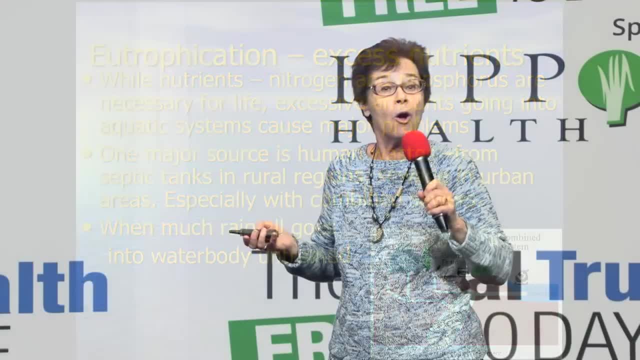 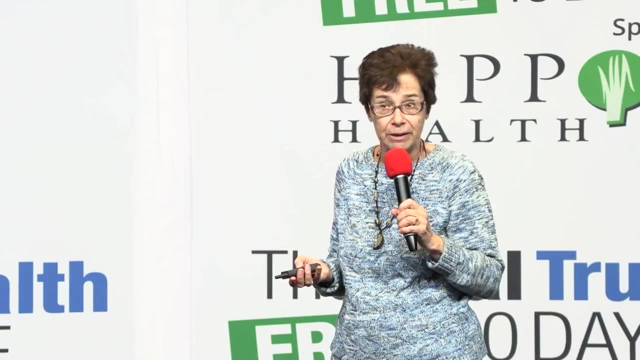 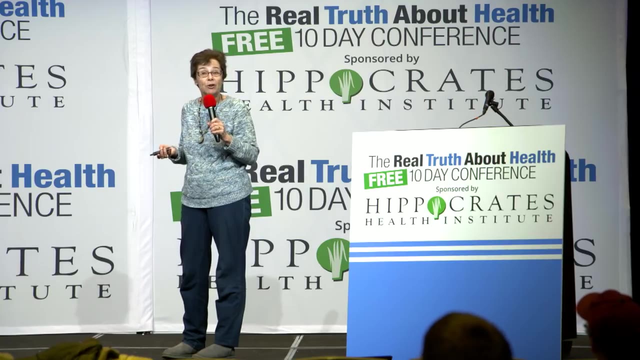 these sewers and together it would go to the sewage treatment plant, which worked fine for a time. it worked fine for most of the 20th century, but during that 20th century the population living in the city grew enormously and so that the amount coming down from the homes and businesses was a lot more than it used. to be, and the sewage treatment plant had a certain capacity that it could take, and it began to be such that on a dry day everything was fine. but if you had a lot, not even a whole lot, a moderate amount of rain, you'd get all this extra water coming in. 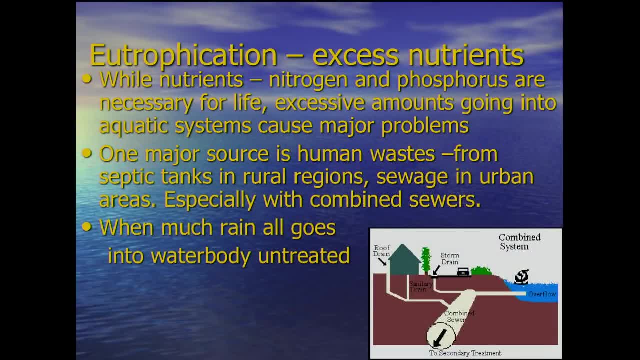 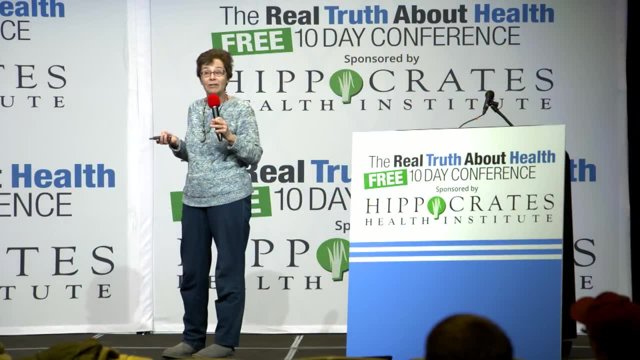 from here, in addition to all this water coming to the sewage treatment plant. and it was too much for the sewage treatment plant to cope with. it had a certain volume of water it could deal with and now it was too much because the population had grown so much. so when it can't go into the sewage treatment plant, it backs up and 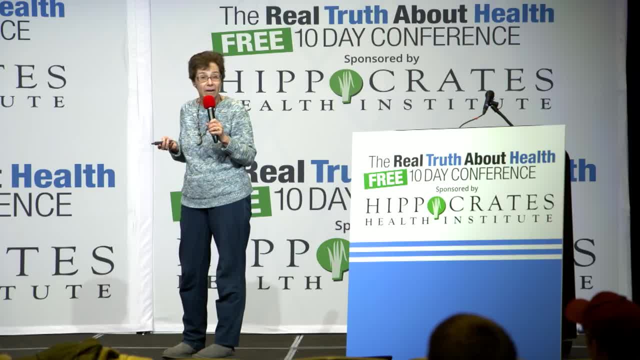 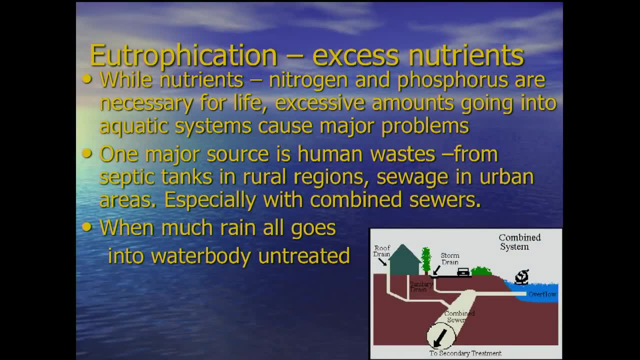 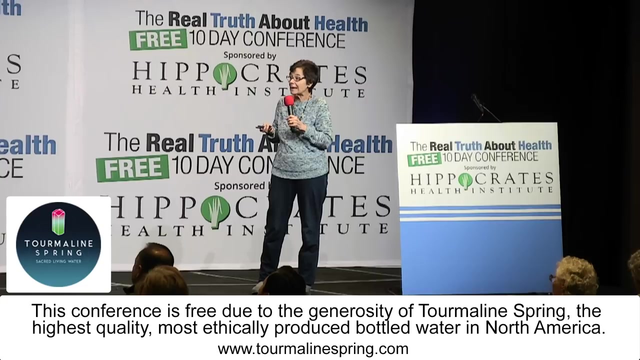 instead of backing up into your toilet or your bathtub, they decided to put an extra pipe here so that it could all go back out to the water. so what that means is that on a moderately rainy day, it overwhelms the sewage treatment plant, and so that sewage, as well as the stormwater, go directly out into the. 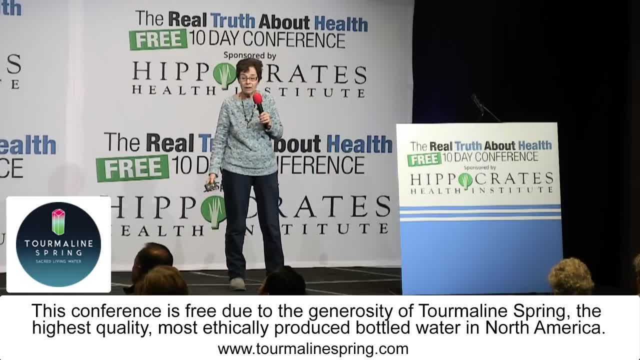 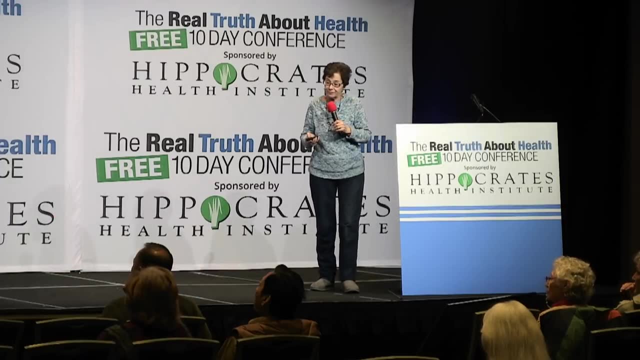 water without treatment. so that's what they call combined sewer overflow and it's the major problem- nutrient problem in urban areas. combined sewer overflow- okay, and that's you know. it's not very pretty to look at when this is happening. this goes into: it's in the Hudson River, it's in the East River, it you know it. it doesn't have to have an enormous amount of rain to have combined sewer overflow. okay, there's also sources from agriculture. the agricultural sources are primarily fertilizer and animal waste, and and the amount of animals used on a large big-ag fire is far more than the land there can absorb the manure. so 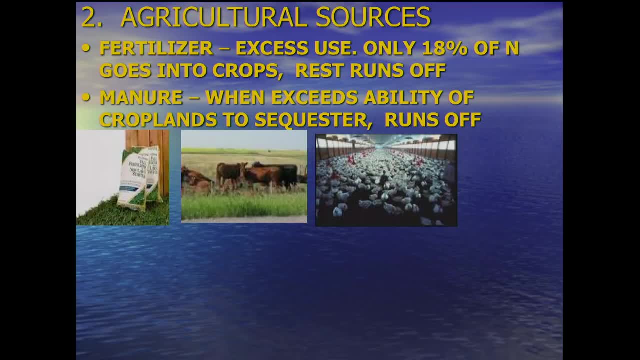 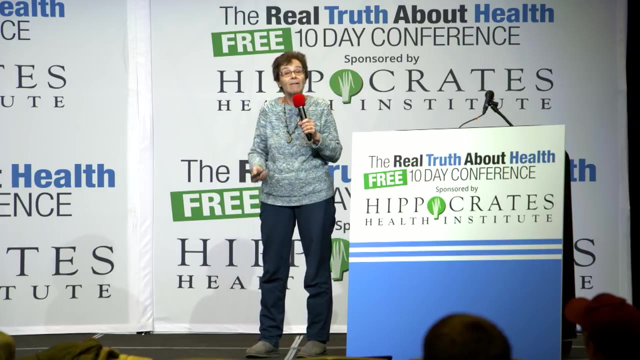 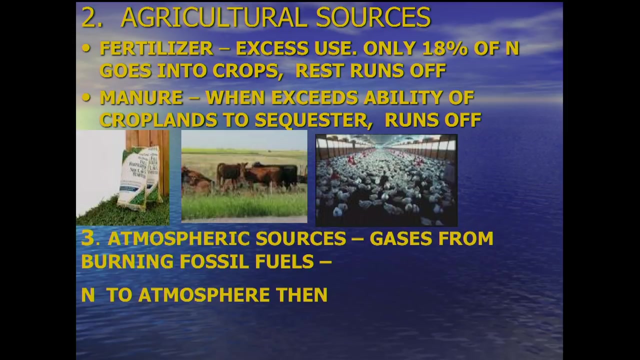 there's a lot of runoff manure into creeks and what goes into creeks goes into streams, goes into rivers. The estuary in the ocean is at the end of all of this, So it runs off. There's also atmospheric sources When you have burning fuel, gas oil. 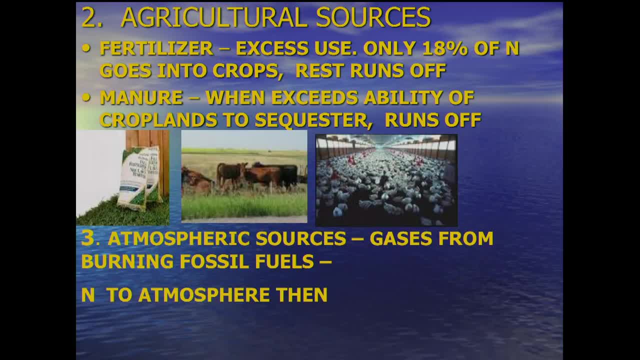 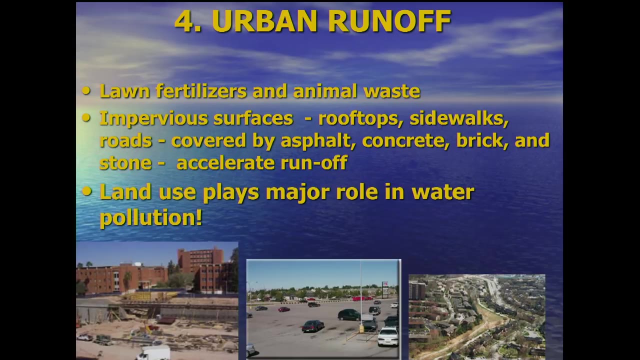 whatever gases from fossil fuels go into the atmosphere and eventually will come down in the rain And when it comes down in rain gets deposited on land and in the water. Another source is urban runoff, Lawn fertilizers and such- I should say urban. and suburban runoff and when it rains- and rain is era- is hitting impervious surfaces, that's roads, sidewalks, parking lots. it can't sink into the ground the way it could if it's hitting open land, park land, forests. 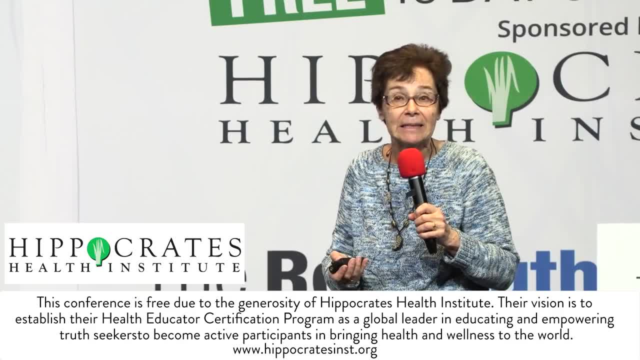 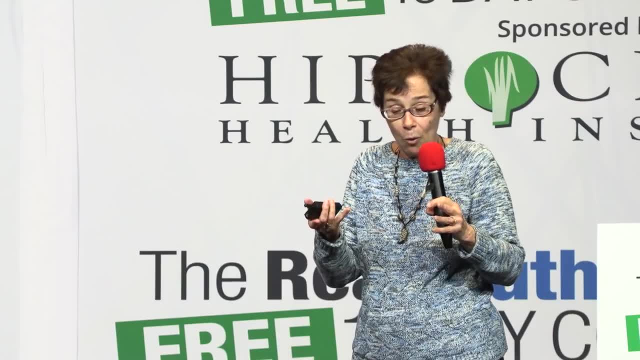 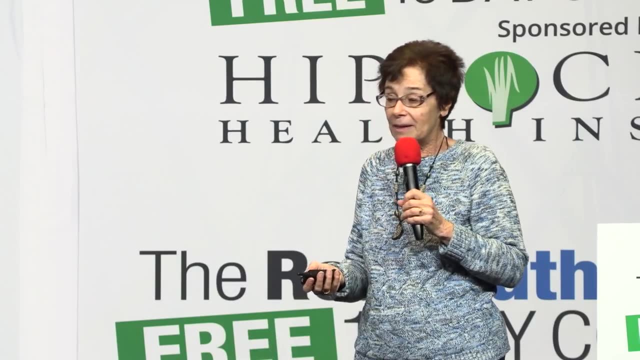 grasslands, whatever The impervious surfaces that are predominant in cities and suburbs, prevent the water from soaking in the land, so it runs off and it picks up pollution on the way into the water. So the take home message here is that land use 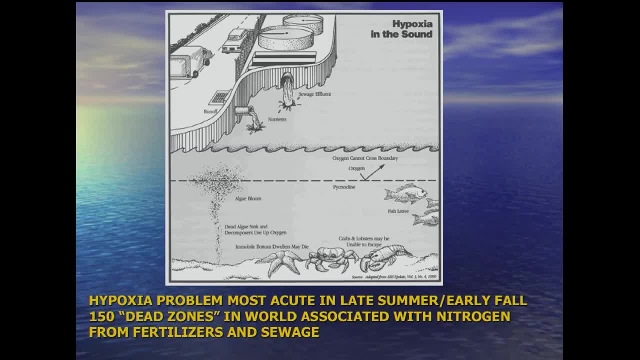 plays a big role in water pollution. Okay, now we get to the thing of. so what does it do? What it does here's your inflow of runoff and sewage into the water. it stimulates, as nutrients will do, plant growth. 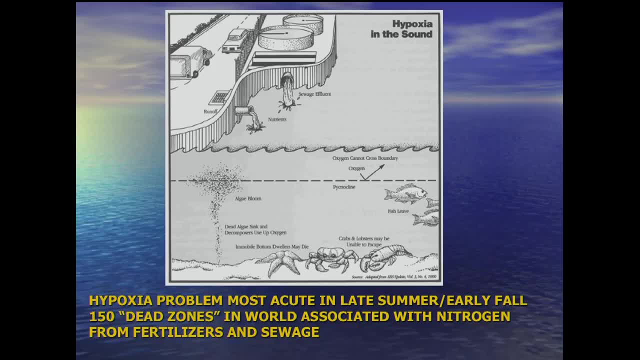 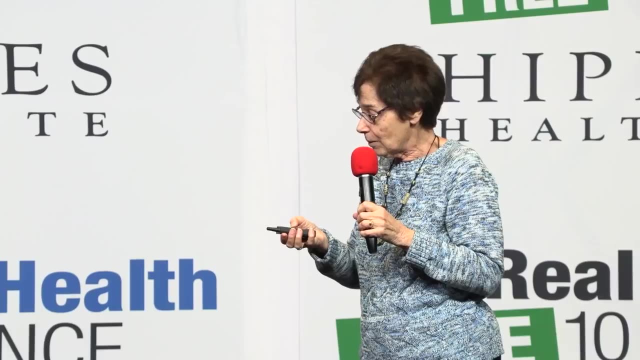 And we're talking here about growth of tiny single-celled plants called phytoplankton or single-celled algae. They get fertilized by this and they grow And you get a bloom. sounds very good, A bloom, right? Well, but whoops, in too much. 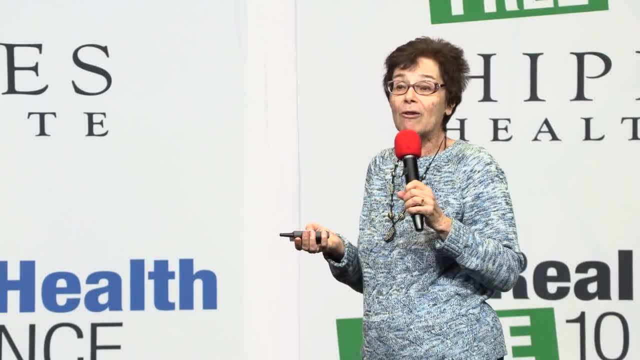 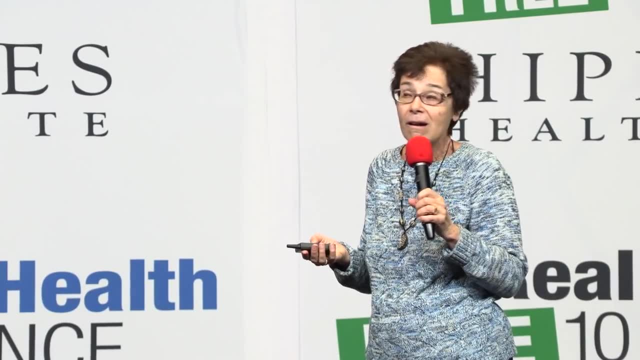 nutrients means too big a bloom. it may grow so much to discolor the water. And if you look at the water, if you look at the water and it looks like pea soup, you know there's something wrong. And here you've got a situation where algae 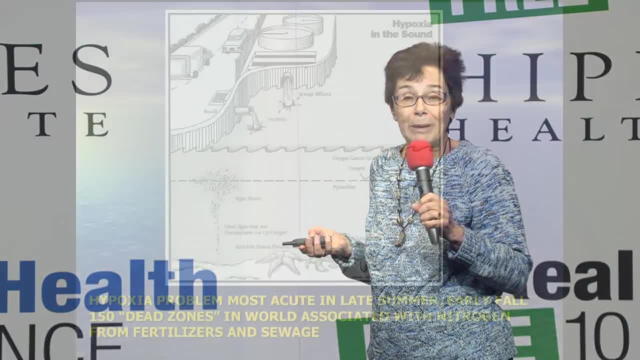 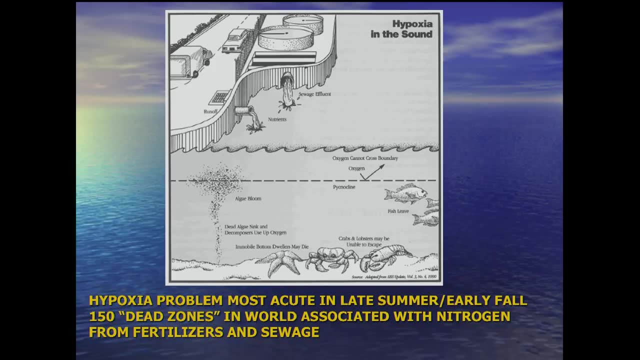 are blooming out of control And this big bloom can't sustain itself and they eventually die. So here we have the dying algae sinking to the bottom. They sink down to the bottom and then they are decayed. Bacteria cause decay And bacteria, in doing the decay, use up oxygen. 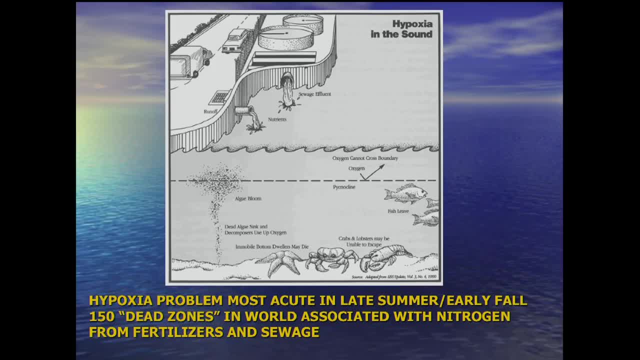 So we end up with a problem that we call hypoxia, which means low oxygen. And that's what? why does this keep blinking? I don't, I'm not doing anything, am I? Anyway, it keeps it down in the lower water. 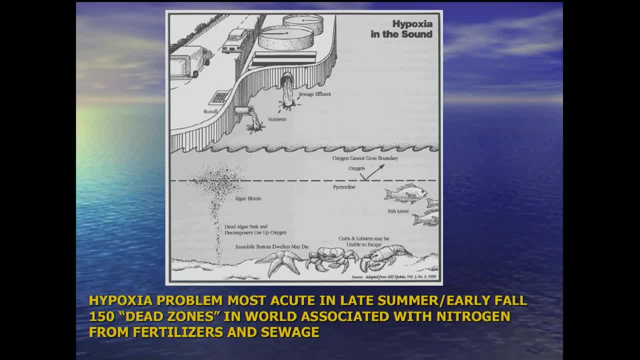 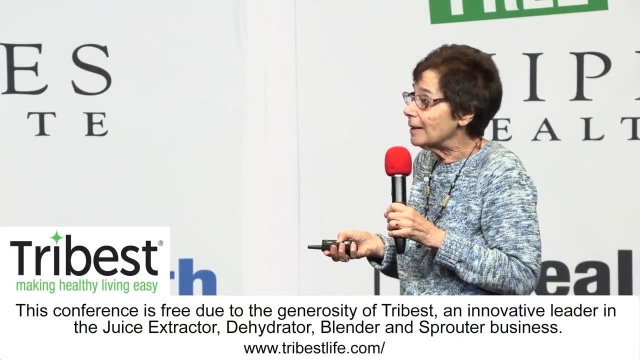 the oxygen goes down, The fish will leave, if they can go, and hope to find someplace where the oxygen is better. The slower moving animals on the body, the more oxygen. the more oxygen, the more oxygen. The bottom may not be able to get away and may die. If it's not low enough to cause them to die. they're still in bad shape, They can't eat well, they can't move well, they can't grow well, So it causes a great deal of damage. That's low oxygen or hypoxia. 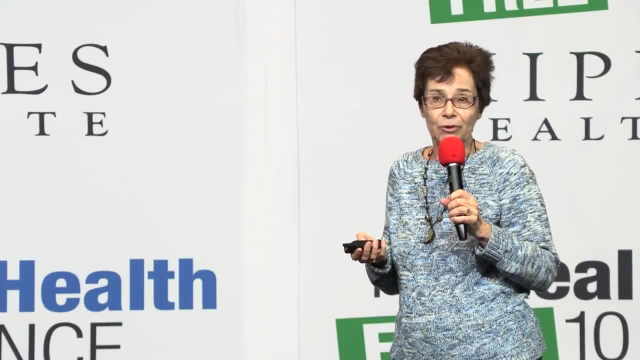 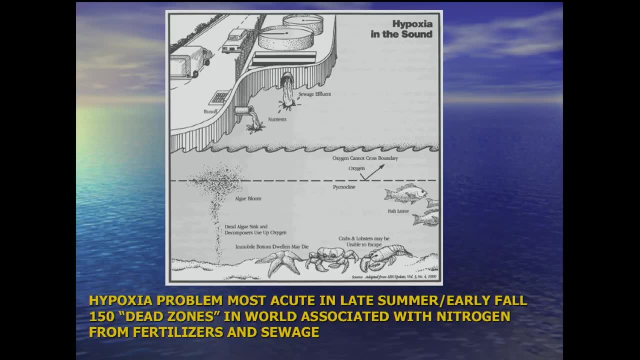 There are areas that are called dead zones that are around the ocean that are often not alive- That's a problem the world- and they're associated with excess nitrogen from fertilizers and sewage coming into the area. the biggest of these dead zones in this country is 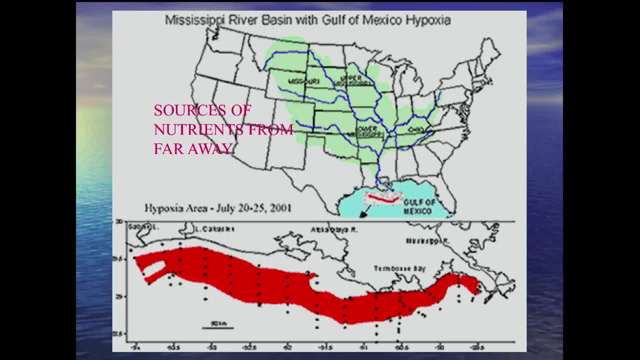 in the Gulf of Mexico and you can see on the map the little here it is, big here it is. on the map they refer to this. they call it. some years it's the size of Massachusetts, some years it's worse, it's the size of New Jersey. and this is a 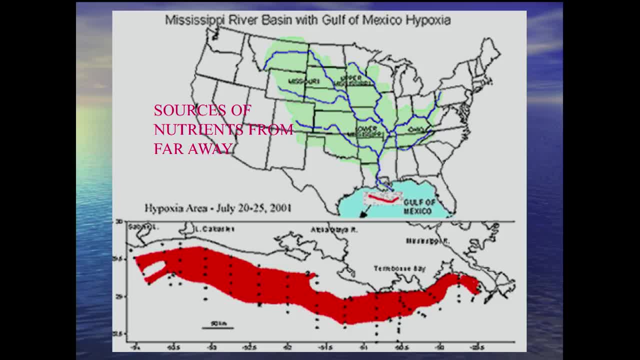 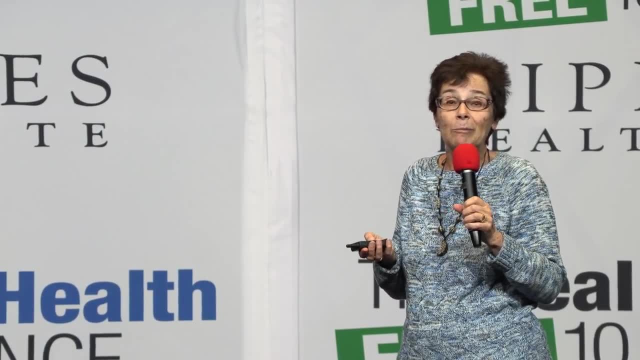 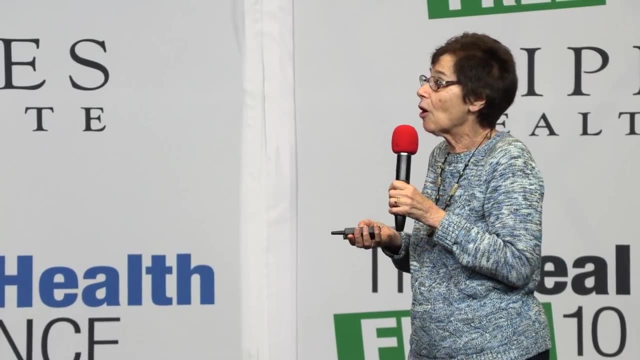 vast area of the ocean or the Gulf of Mexico where there's not enough oxygen for most life to exist. there may be just some bacteria, but you won't find fish. you won't find other other marine animals living there, because the oxygen is too low. now why is this one so bad? you think of what's 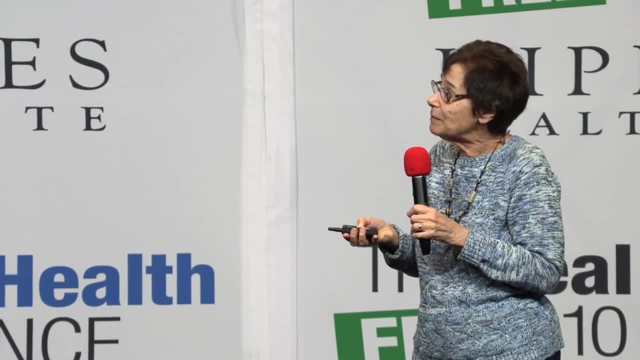 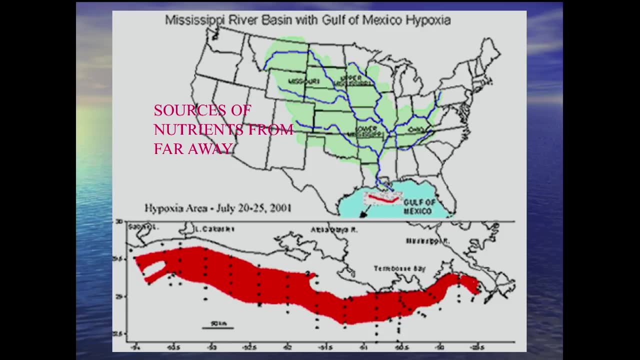 coming into the Gulf of Mexico. we have the Mississippi River coming into the Gulf of Mexico. the Mississippi River is receiving tributaries from all of these states. this is the breadbasket of the US. this is the big agricultural area of the US. these rivers and streams are loaded with fertilizer that's runoff from all. 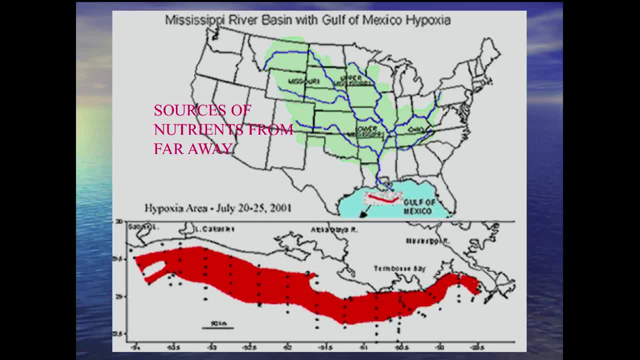 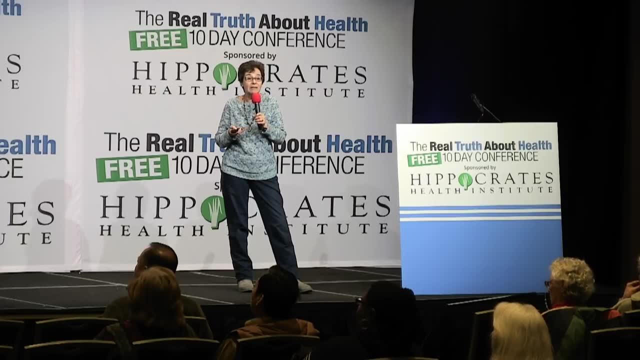 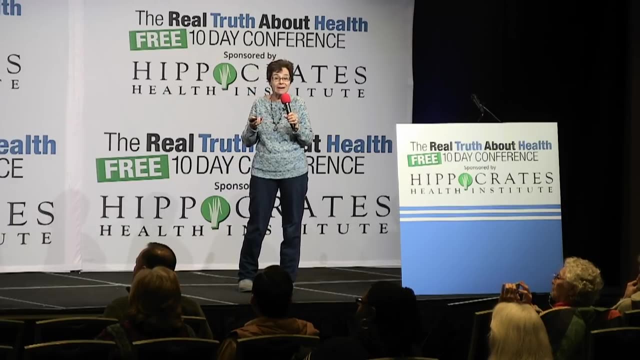 the farms, it's coming together to the Mississippi and getting dumped into the Gulf of Mexico and hence you have this large dead zone. the dead zone is largest in years. with a lot of rain, it all comes back to rain and runoff of the fertilizer. on a dry year, you have less rain, less runoff, a smaller dead zone. 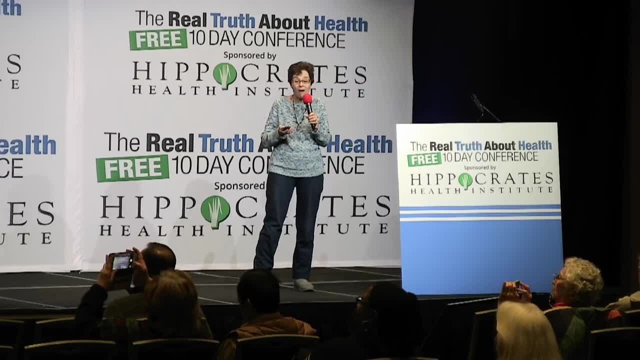 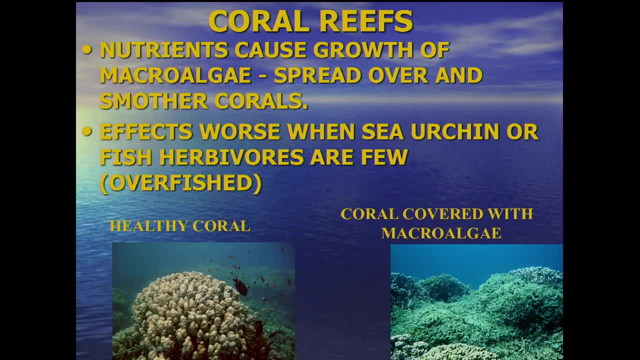 not near us. further south we have coral reefs that are also in big trouble because of excess nutrients and its eutrophication. The excess nutrients cause other kinds of algae to overgrow the corals and cover them. And you see, on the right side here. 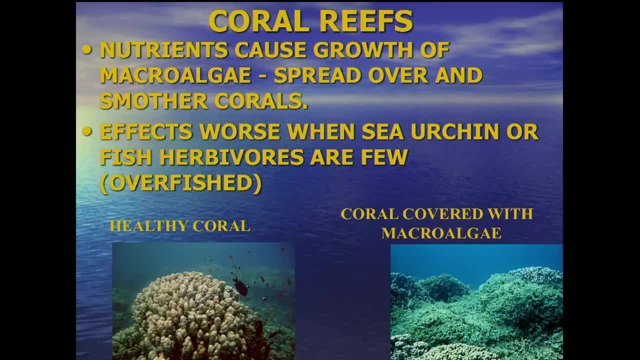 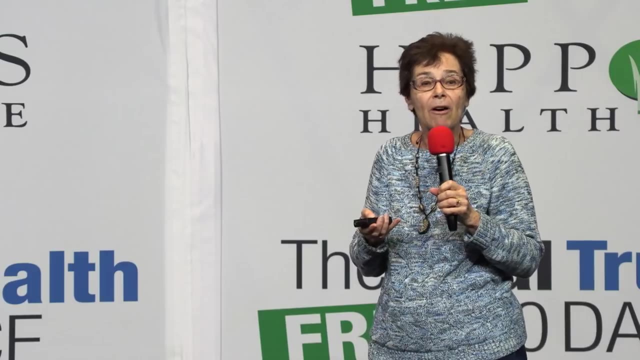 it's green, bluish green. That algae has covered that coral. This is what the coral looked like originally. Here it is covered with algae because the algae was stimulated to grow by the nutrients coming in. If you have a lot of animals around that eat that algae- things like sea urchins- 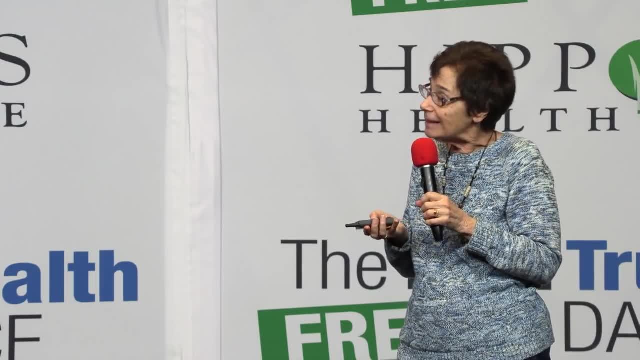 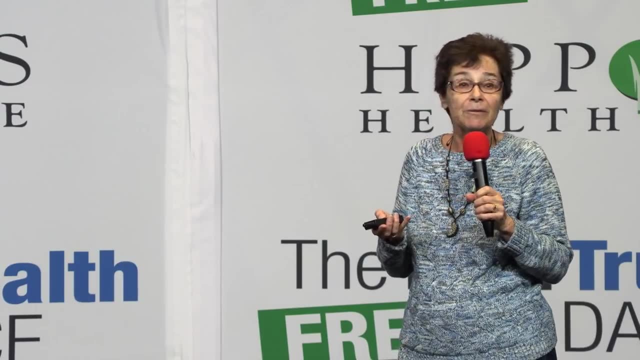 things like certain species of fish could eat that algae. they may be able to keep the thing under control, But if your fish are in bad, if you've overfished, for example, and you don't have many of those fish around, 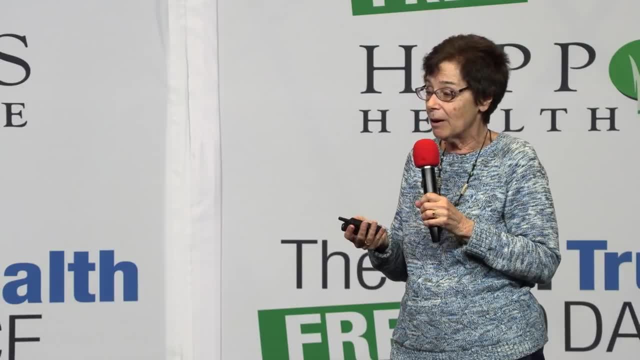 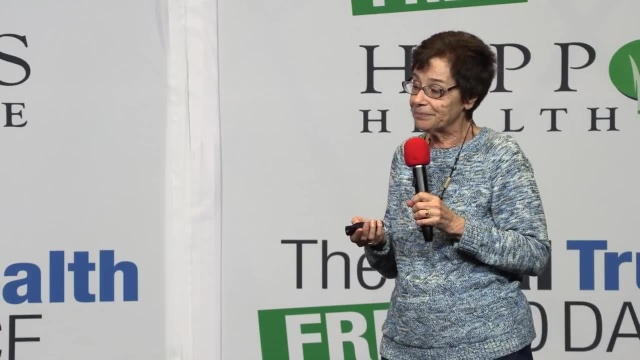 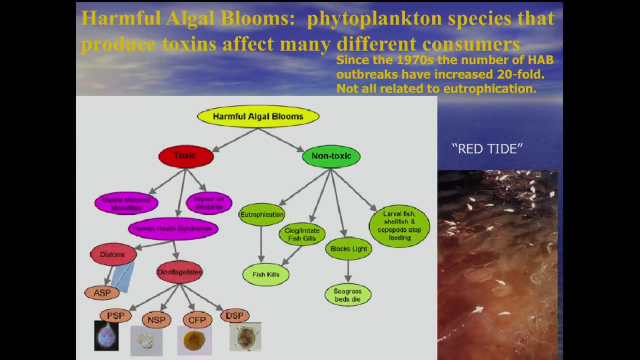 then your coral reef is in trouble. They're in bigger trouble from getting their algae overgrown, getting the coral overgrown by algae. Another problem that happens with algae, in this case certain species of single-celled algae, is that certain of these species produce. 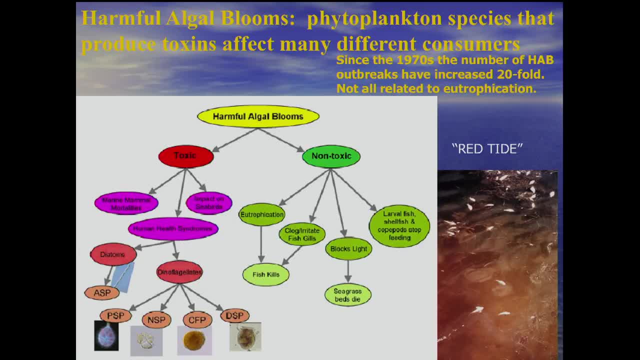 toxins, And they're the ones on the left side here. There are certain species of single-celled algae that produce toxins that may either be released into the water and cause problems, or may only cause problems for animals that eat these algae, And they're showing in this picture several different ones. 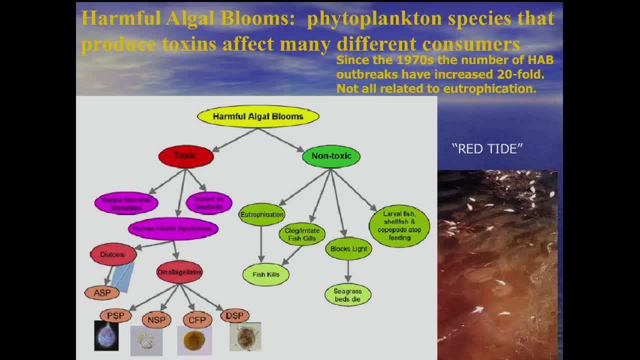 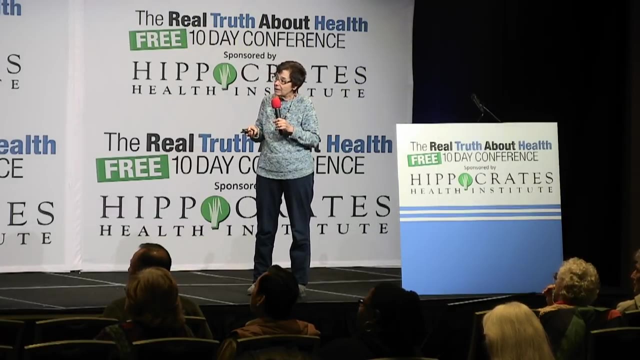 There are many more And as time goes on, people keep finding new species that are producing these toxins that are harmful. There are. there's one that happens around here- That's the one here. It's called PSP- paralytic shellfish poisoning. 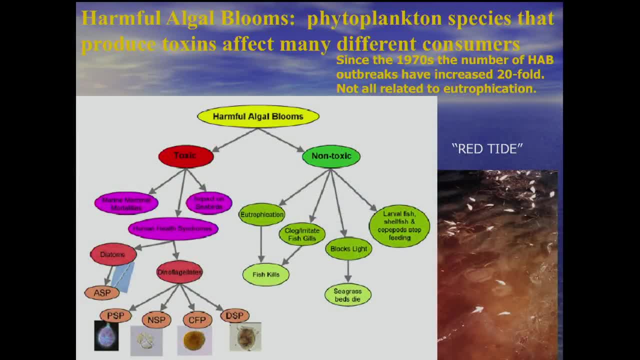 Why shellfish? What happens is shellfish, like clams and oysters, will eat their filter feeders. The water gets pumped through their systems and they filter out algae from the water. And if these toxic species of algae happen to be around, 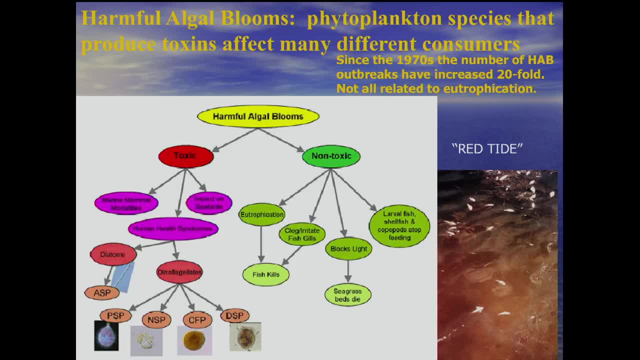 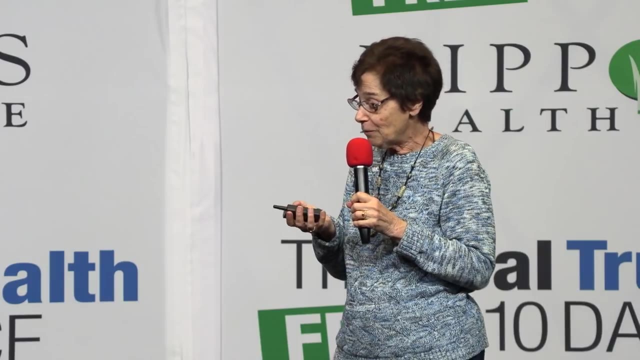 they eat them just as much as anything else And they can store the toxin in their tissues. It doesn't kill them, It impairs them somewhat, but they can survive And they can manage to store up pretty high quantities of the toxin from these algae. 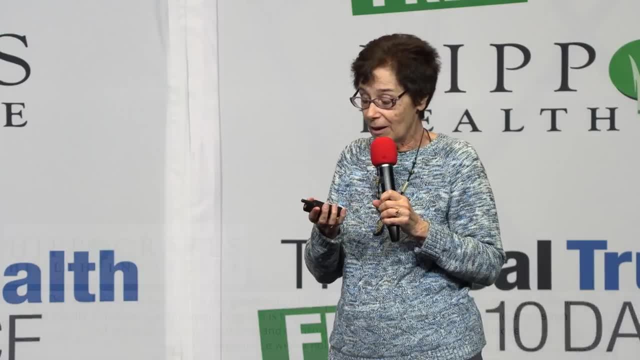 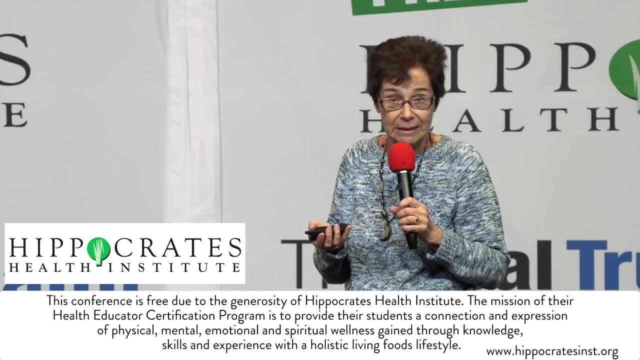 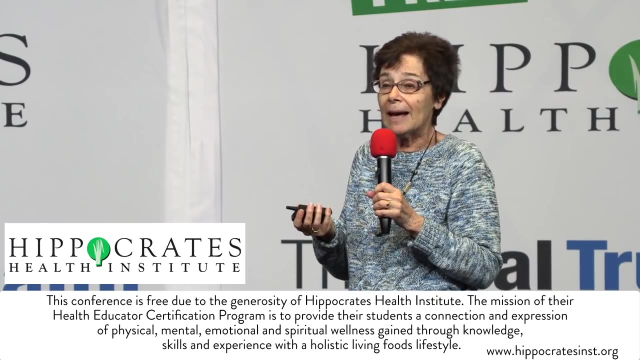 And then if you or any unlucky person should happen to eat some of those oysters or clams or mussels, then you get very sick. So this is a human health issue. What is done is that the beds of these shellfish that are harvested for people to eat. 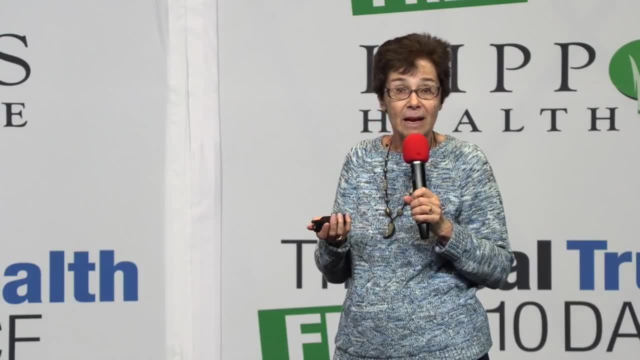 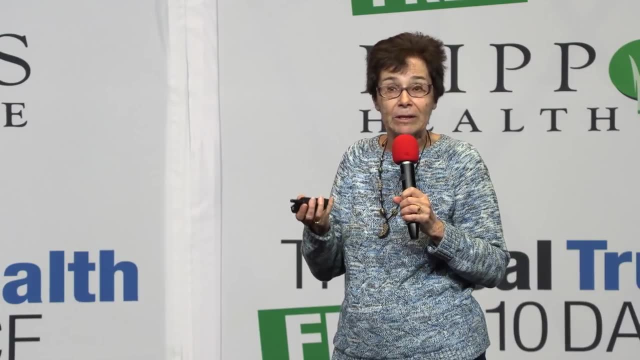 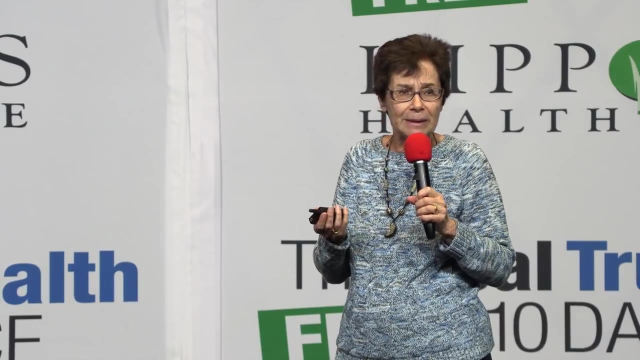 are monitored regularly and tested to see if these toxins have been accumulating there or not And if, if they find over a certain level of the toxin from these algae, they will close the bed, So that very few incidents of paralytic shellfish poisoning happen, but there are. 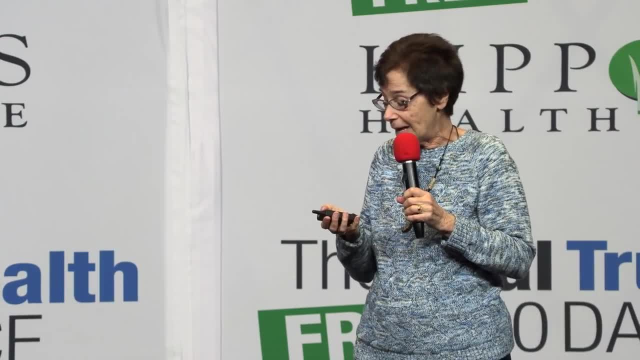 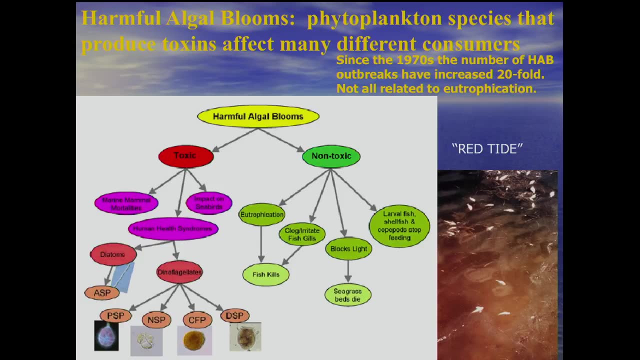 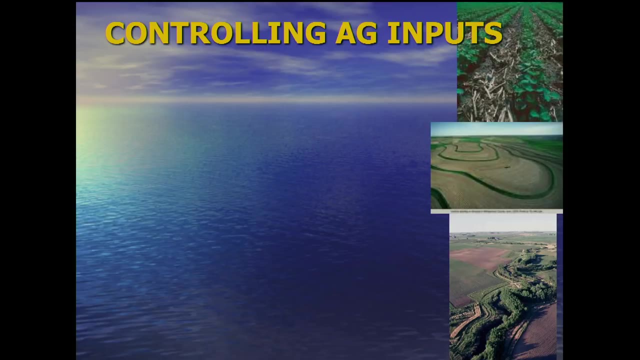 some of these other species that are rarer, and people have died from eating too much shellfish that have accumulated some of these toxins. so now the next part is: what can we do about it? well, we can reduce the input of these nutrients- nitrogen for example- from agriculture. there are various 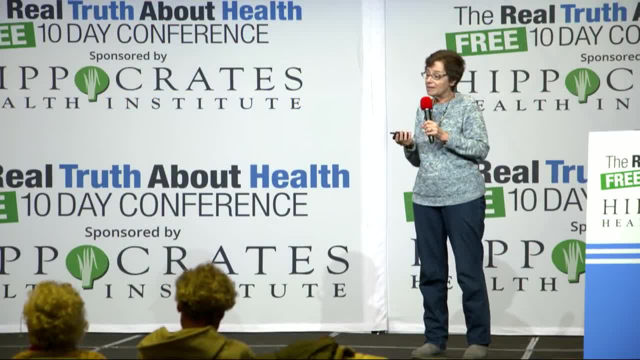 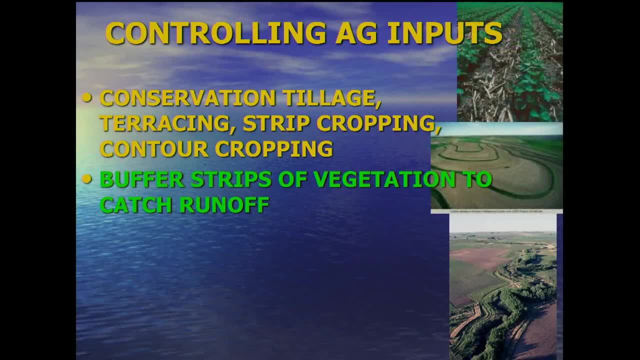 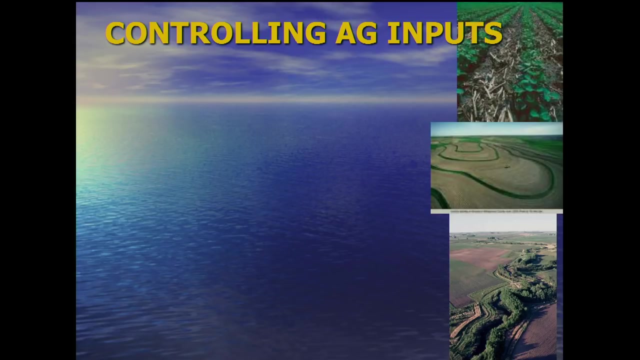 agricultural techniques: conservation, tillage, terracing, contour cropping. here's an example here. oh, I'm pushing the wrong button, I'm sorry, let's. let's go back a little bit. this picture here: you see that here's a creek going along here at here is some crop, some shrubbery growing right at the edge of the creek, and 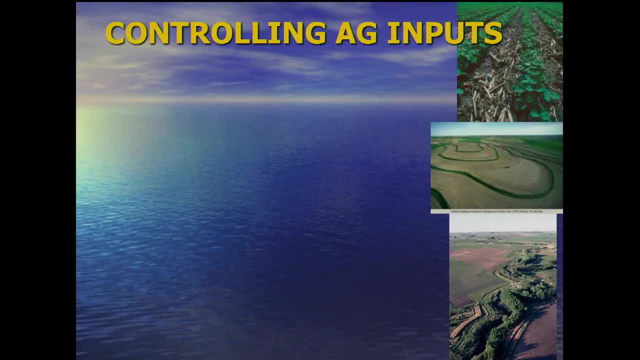 here's the farm field. so what they did was they planted this plant so that when there is rain and runoff, this is, this is not the crop, this is trapping the nutrients that are running in and preventing them from getting into the creek. so things like that, and there's a whole slew of them that have been known. 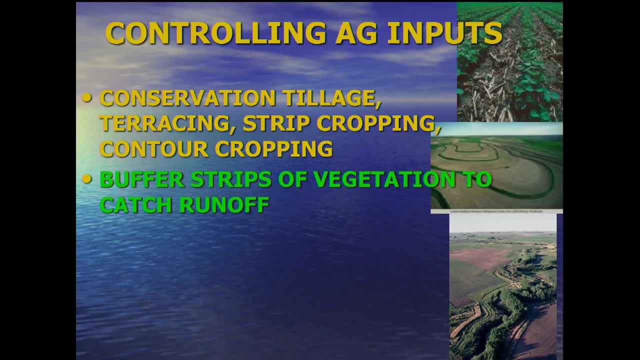 and done for many years. that's called a buffer strip of vegetation and it catches the runoff and prevents it from getting into the creek. of course it's also possible to reduce the use of fertilizers. farmers tend to use far more fertilizer than is necessary. a small fraction of the fertilizer actually gets into the plant. 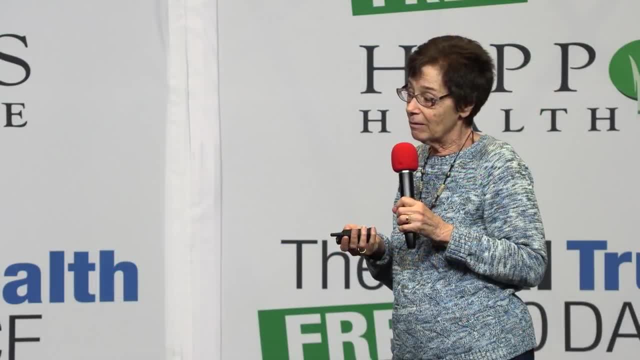 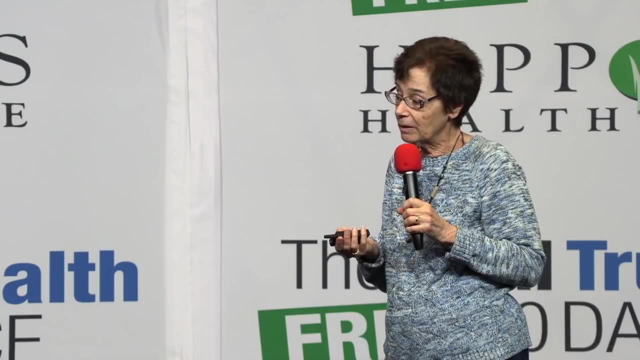 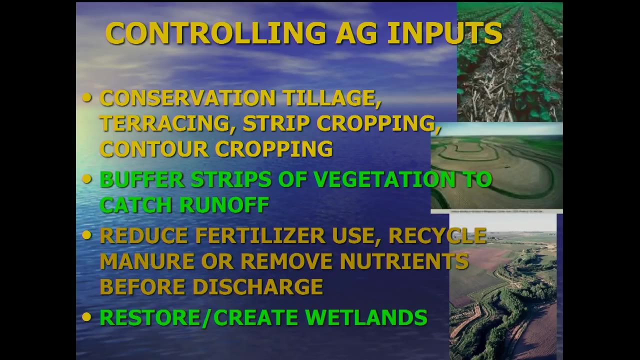 and and more than half of it ends up running off. so there are many things that farmers can do. the problem is it's all voluntary. another thing that can be done is restoring or creating wetlands that will also serve as a larger than that buffer strip, but the same idea: the wetlands. 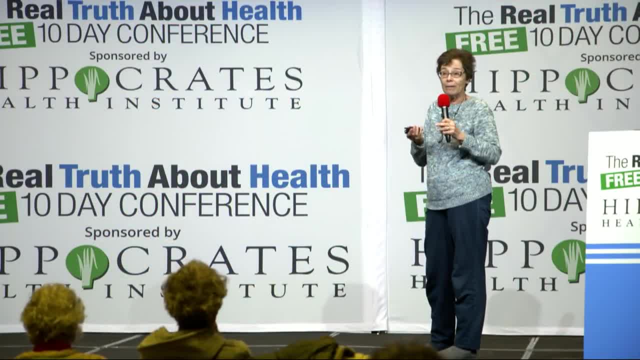 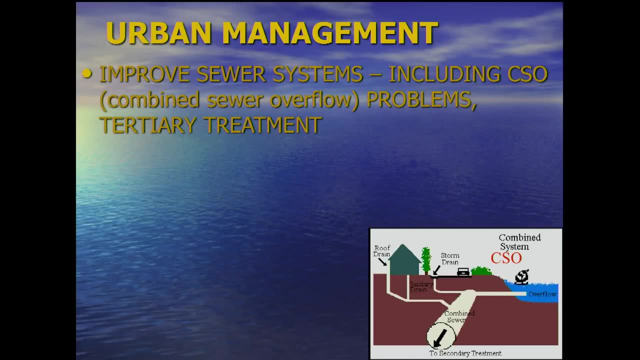 will absorb the nutrients and help the wetland plants grow, instead of going into the water body and causing utrophication. urban management: what can we do about this sewer problem, this combined sewer? well, it's a very bad thing. it's possible to do tertiary treatment to improve the sewage treatment also. 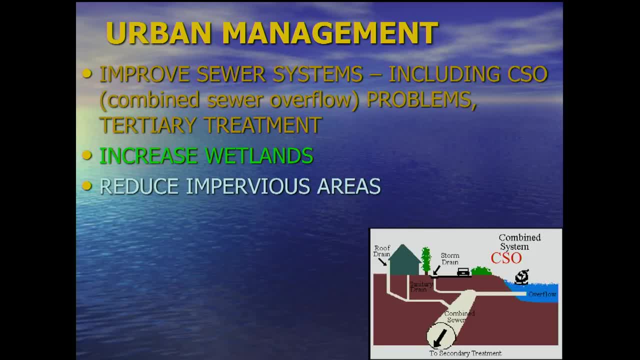 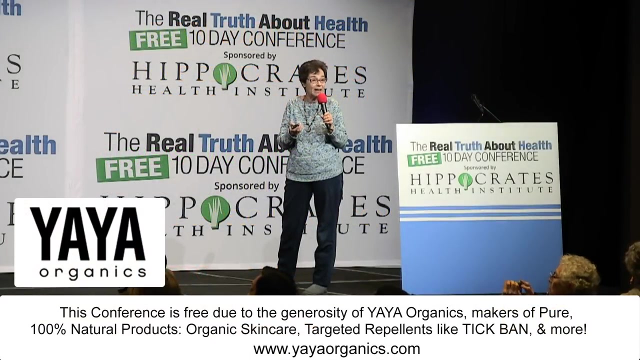 wetlands, reduce the amount of impervious areas, reduce erosion from construction sites. and the thing that has become quite popular these days and really needs to be magnified greatly is storing stormwater. if you can have less stormwater running off into the storm sewer and collect it somewhere and hold. 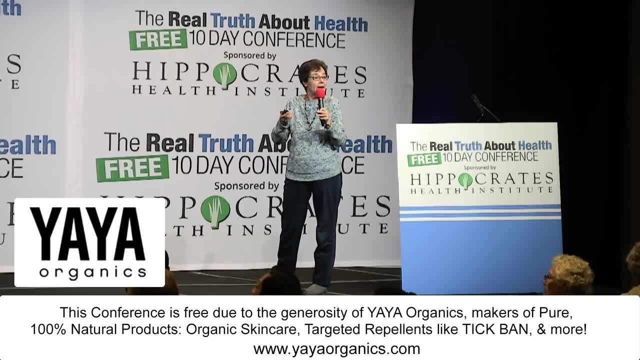 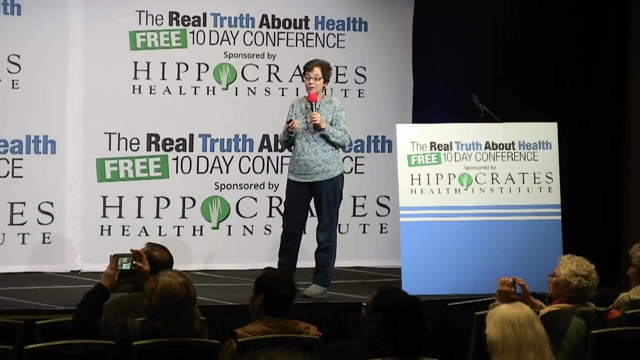 it and then slowly, after the rain is over, slowly feed it back into the system. this would solve it if you could make some large humongous pool somewhere to just hold it. but there were even better ideas. there's green infrastructure and there's a bunch of these things that are referred to as green. 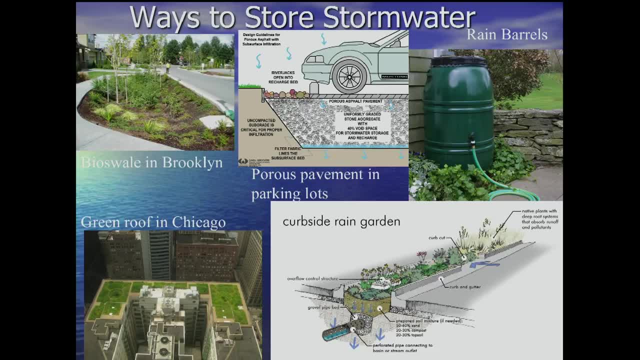 infrastructure, infrastructure. They can make things like bioswales or rain gardens. This is just dirt and plants instead of concrete, instead of asphalt. So here, these bioswales are put near curbs on streets and it's greenery, It makes it prettier and it absorbs a lot of the water. 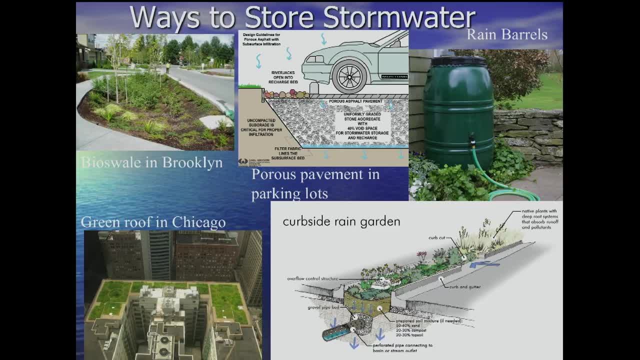 that would otherwise have washed down the sewer into the water. There are rooftop green roofs and we have one in New York City on top of the Javits Center, which is a big convention center on the far west side of Manhattan. Then smaller scale rain barrels. People can have a rain barrel. 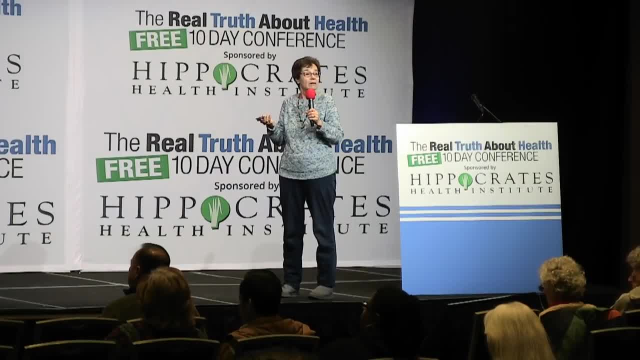 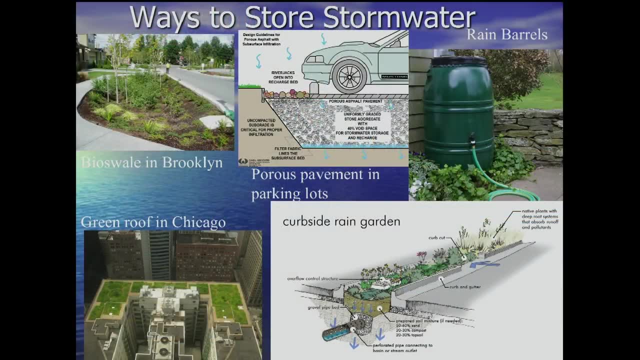 in their garden and then tap off the water to water their garden the next week when it's not raining. And there's also this thing called porous pavement, which is a constructed thing which will absorb a fair amount of water, instead of the normal pavement that absorbs no water. 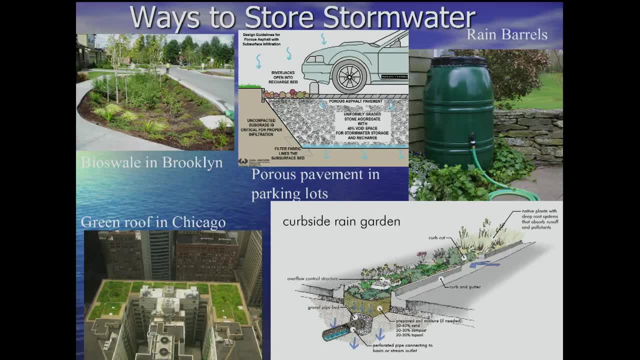 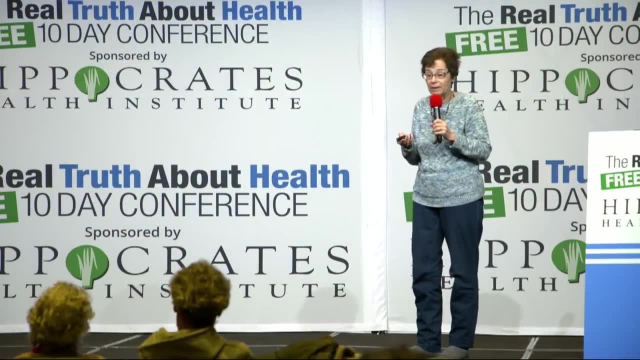 And then it stores it for a while and then feeds it back to get back into the watershed. So there are lots of ways to store stormwater And New York City is doing a lot of this. They're not doing it as much and as fast as a lot of us would like, but it costs money. 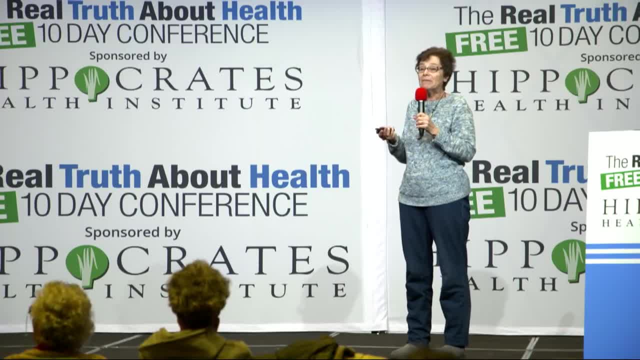 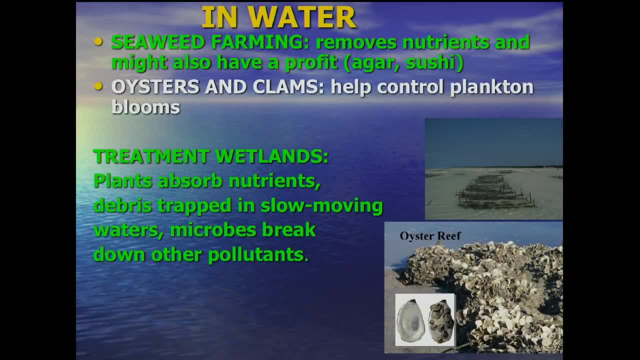 to do these things. Even in the water it's possible to do things to reduce this. You can grow, have seaweed farms Here. this is a seaweed farm. They have some in Long Island Sound, off the coast of Stamford, I think, somewhere in Connecticut. The seaweed will absorb the nutrients and 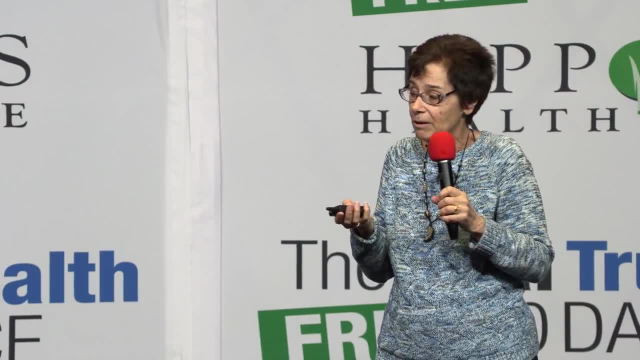 then you can harvest it and use it in sushi or whatever. I don't know. I'm not sure about that, But you can use it to grow food and you can use it for cooking. know other other thing you can think you can do with it also: shellfish growing. 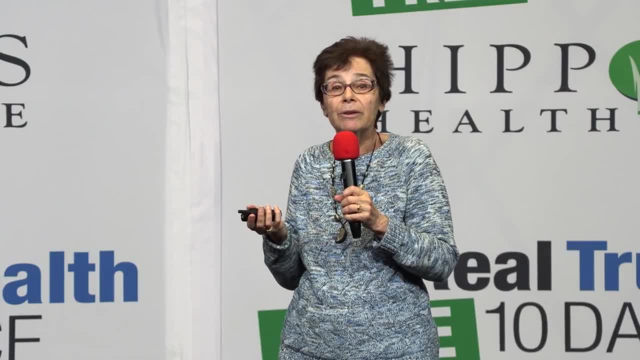 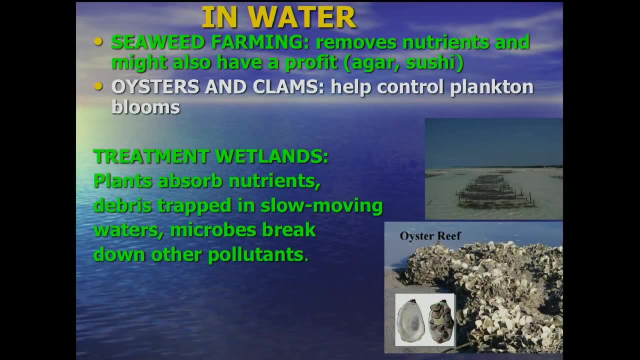 oysters and clams. they're not going to absorb the nutrients, but they will eat some of the plankton that are blooming and reduce the size of a plankton bloom. and then there are also treatment wetlands that will have plants to absorb the nutrients. so even once you're in the water, it's not necessarily too. 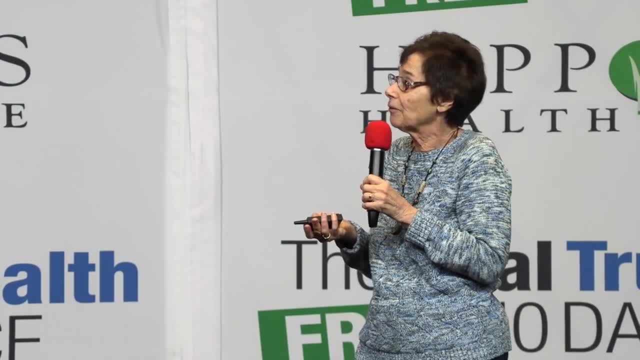 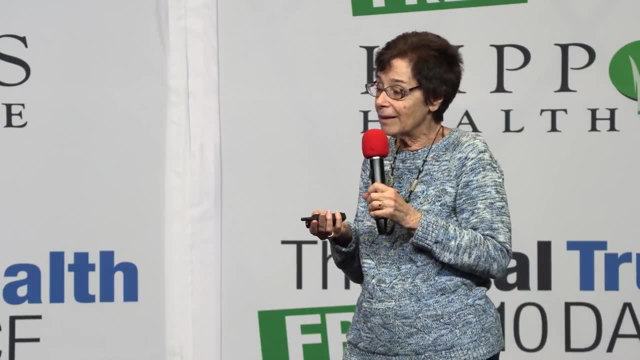 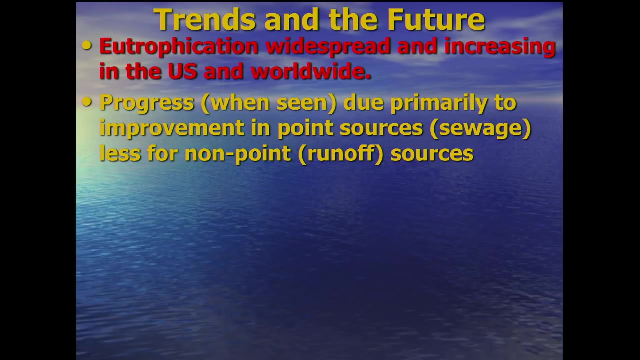 late, it's possible to do something to reduce eutrophication even in systems in the water. overall, things are getting worse. eutrophication worldwide is getting worse in the US and worldwide. areas of progress that we've seen are mostly in terms of improvement of sewage treatment. 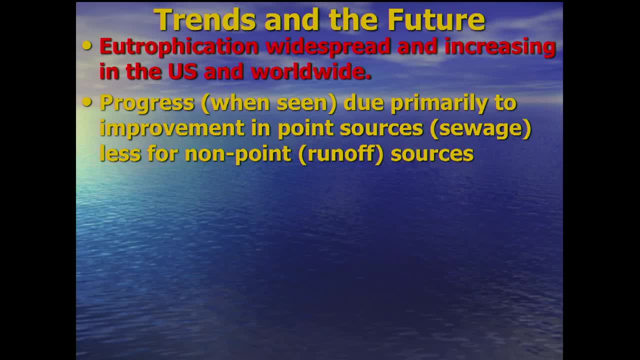 plants and combined sewer overflow issues. there is less improvement on sewage treatment plants and combined sewer overflow issues. there is less improvement on the non-point source runoff, that is, runoff from fields and agriculture, and that harmful algal blooms are increasing in frequency and also they keep finding. 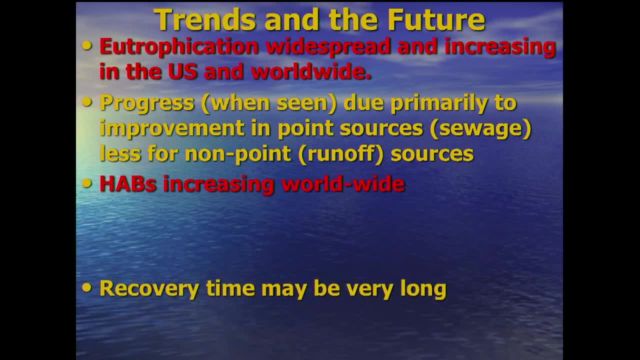 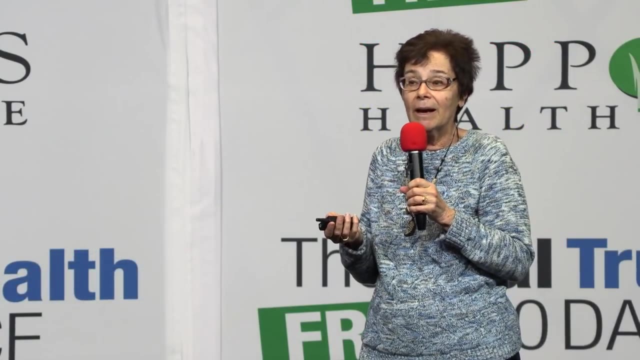 new species that they had not known about before. another thing that makes problem for politicians is that recovery time may be very long. you do something to fix it. the politician may not be able to fix it. the politician wants to see a difference by next year. that's not going to happen. there is a 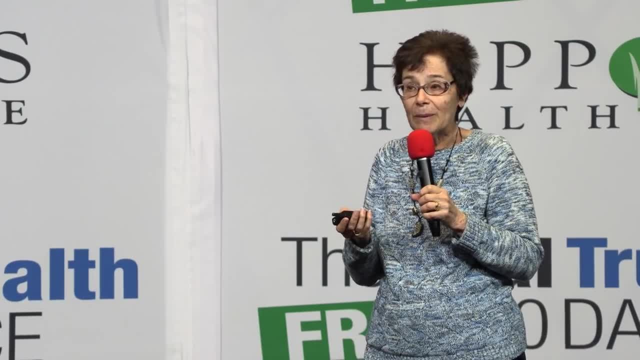 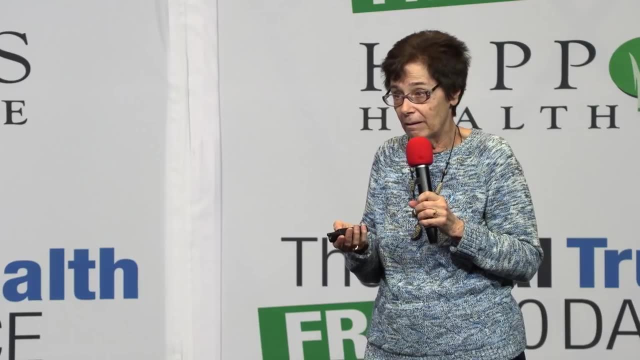 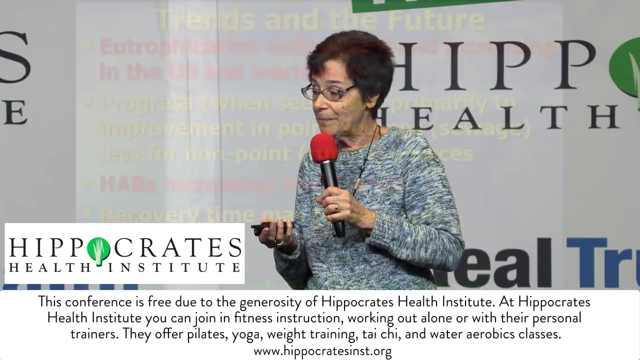 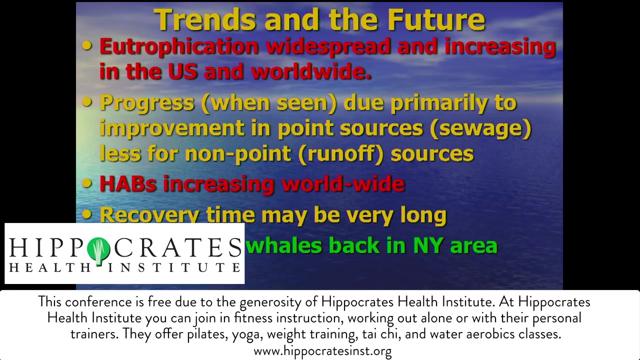 long lag period here, so you can spend a lot of money to fix something and not see an improvement in possibly a decade. so that is a hard thing to convince a politician on, but that's, that's the bitter truth about this. some good news: our oxygen levels around New York are better and we've got whales around New. 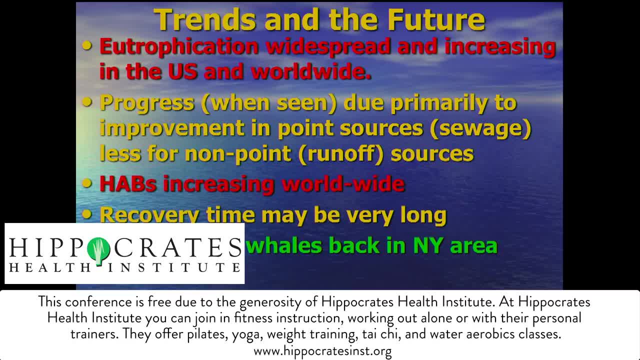 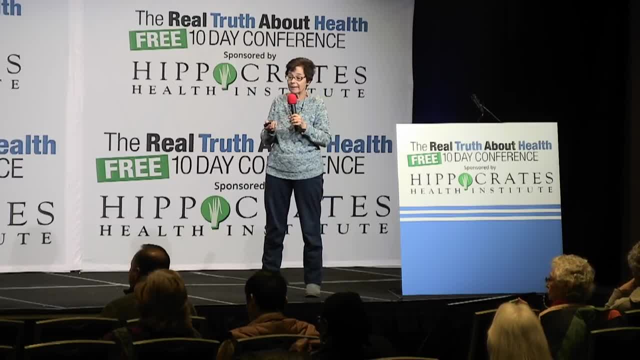 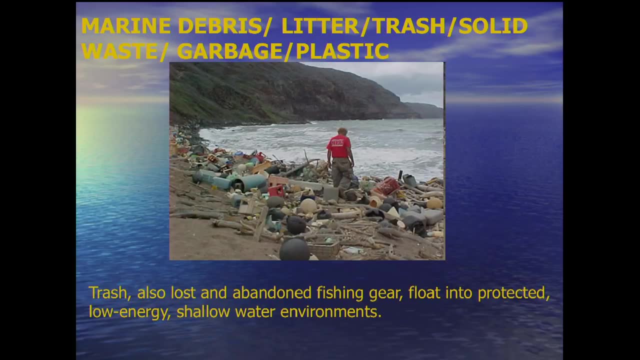 York. so things that were really awful in the 70s and 80s have improved, but things that were really good in the 70s and 80s have gone down. okay, another switching to another type of pollution. it's got many names we can. 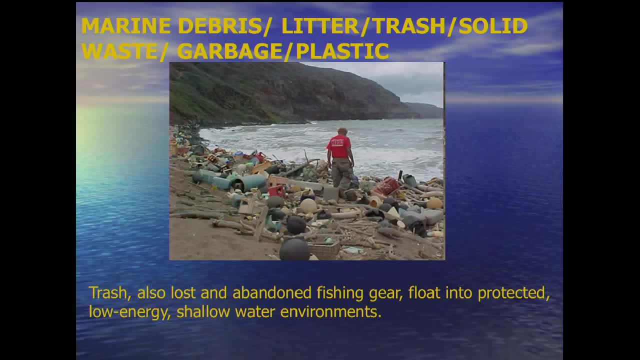 call it marine debris, you can call it litter, we can call it trash, we can call it solid waste, garbage- take your pick. it's all the same stuff and it's mostly plastic. and you've probably all seen pictures like this when I talk about the this, of some beach piled up with litter, debris, plastic, whatever you want to call. 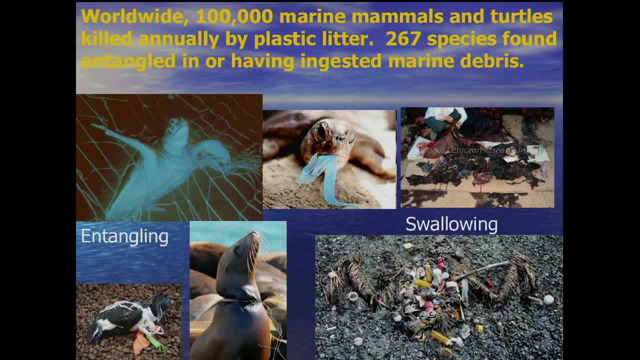 it. it's really ugly. I don't have to convince you how ugly it is. but it's also harmful. it's not just a matter of being ugly: marine animals are getting killed by this stuff. one major way they're getting killed is by getting entangled in it, like this turtle here, or the seal and the bird here. they can. 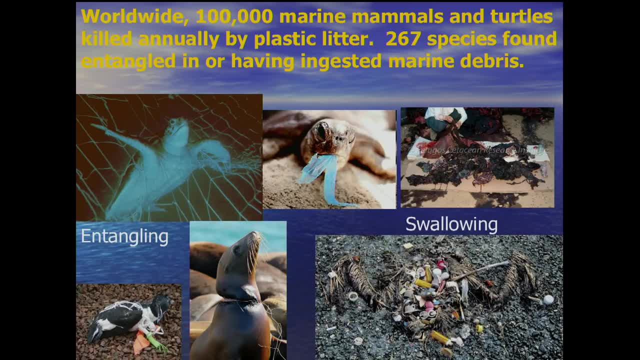 get entangled in the plastic. another way they are damaged by it or killed by it is by eating it, and we've got here a turtle in the process of eating a plastic bag. we have opened. animals have been opened up. I've got more of this later here. this is a dead bird. 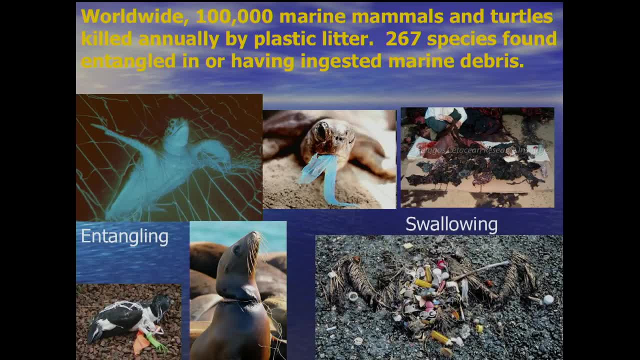 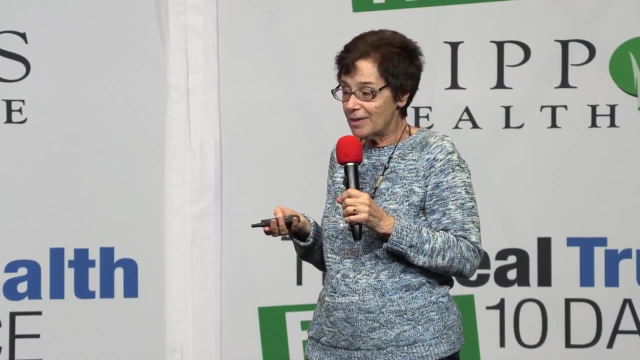 opened up a carcass. you could see sort of the wings here. this is a baby bird and if you look here it's full of plastic. the albatrosses in the Pacific Ocean, the parent birds, pick up plastic and feed it to the baby birds. and who? 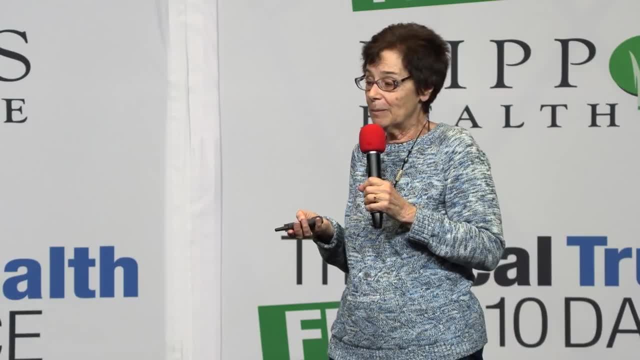 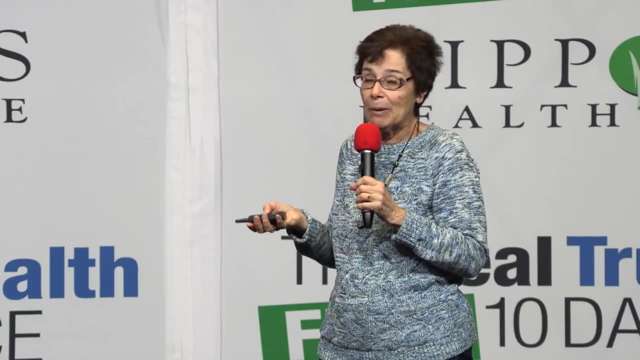 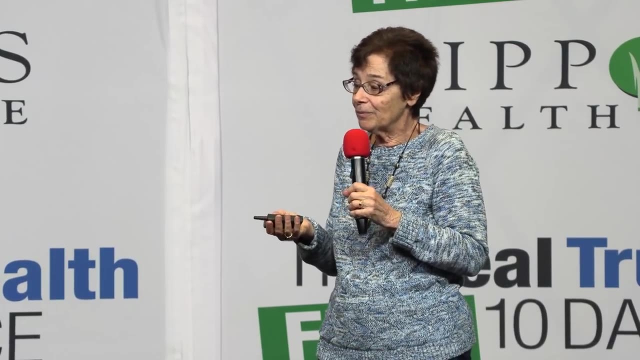 know they don't know any better, and the baby birds don't know any better, and they eat it and they die. I mean, I can't prove to you that this baby bird died from all the plastic in its stomach, but I think we all know it did. I mean, it's kind of self-evident. 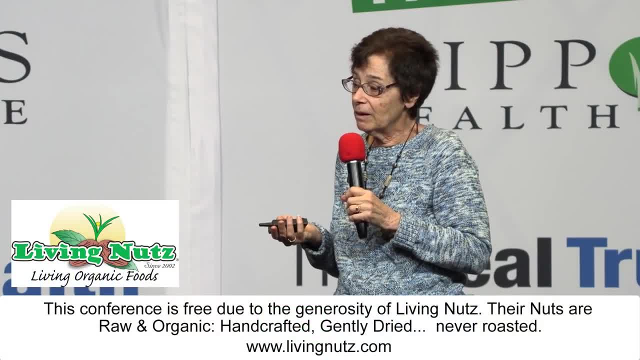 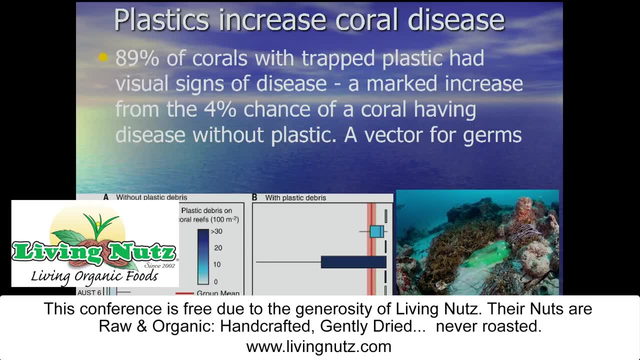 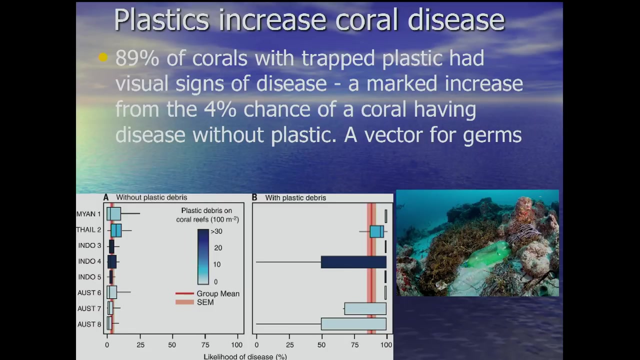 that it did. there's a new paper that just came out last week that Carl disease is much more prevalent when there is plastic litter sitting on the Carl. the litter apparently is a good way to transfer disease organisms, germs. the plastic lands on the reef and that area of the reef has much more disease than an area of the reef. 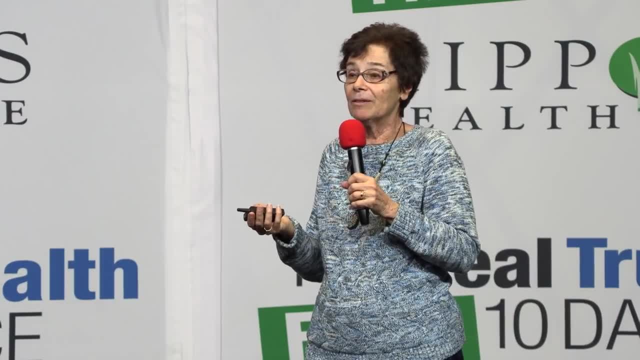 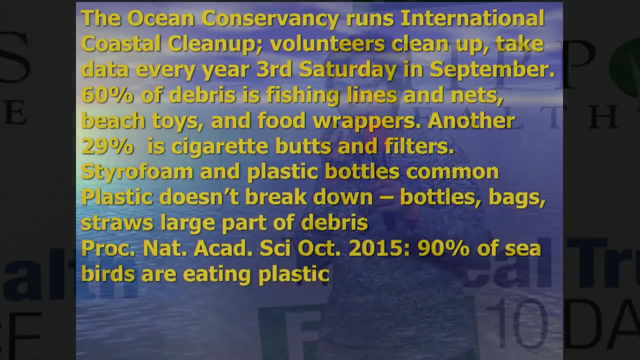 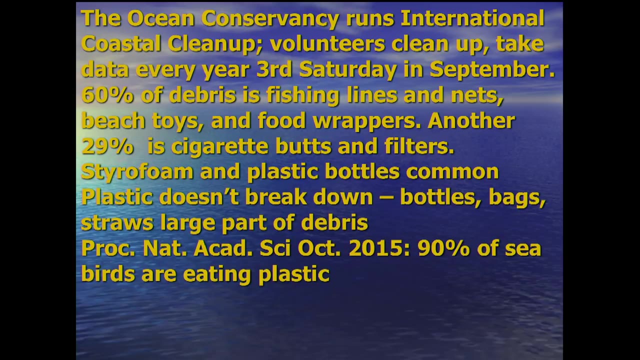 that doesn't have plastic on it. so here's something new, a new way for plastics to kill animals. there is- and perhaps some of you know that this- a international Beach cleanup, coastal cleanup run by the ocean conservation, every year in September. and they don't only just pick up, they keep excellent. 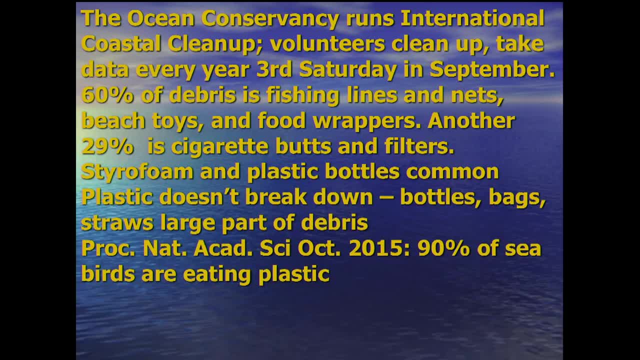 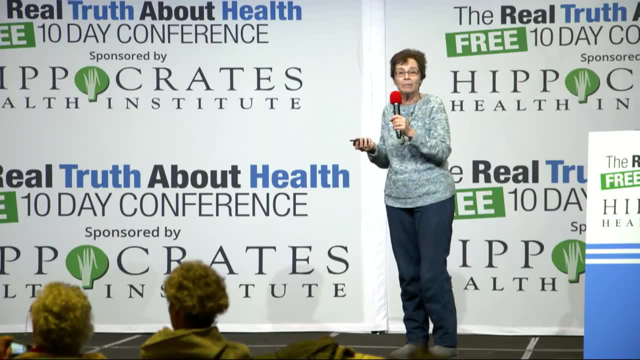 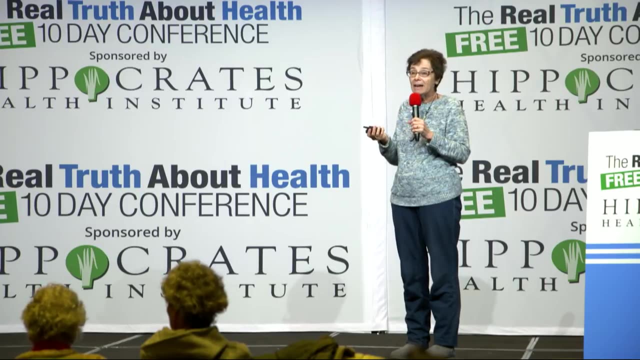 records. so there's tons of data. everyone who goes to pick up stuff on the beach gets a sheet to fill in: how many cigarette butts you found, how many police's of balloon, how many plastic bags, how many bottles and so forth. so they have excellent data over the years and and you find that cigarette butts 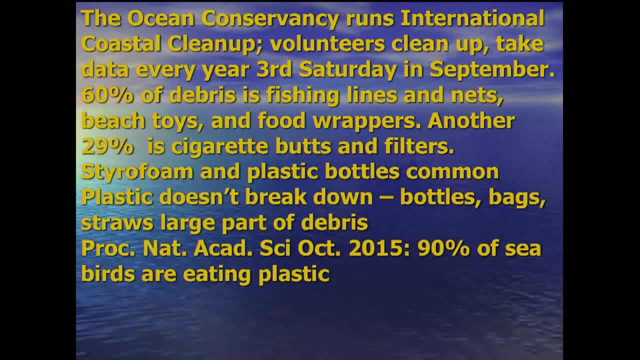 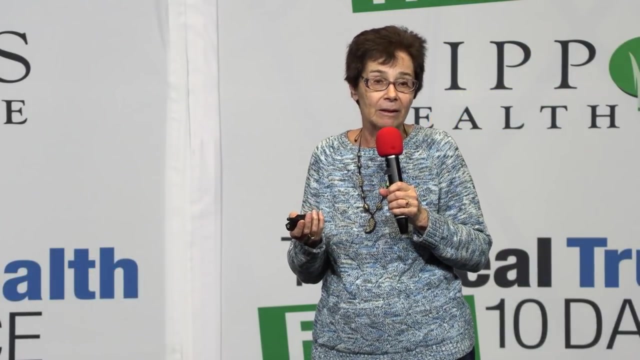 are very common: fishing lines and nets, food wrappers, styrofoam plastic bottles. the thing about plastic is that it doesn't break down. it breaks up into smaller pieces, but it doesn't break down chemically. and then there was a report not that long ago: ninety percent of the seabirds- they look they analog we're. 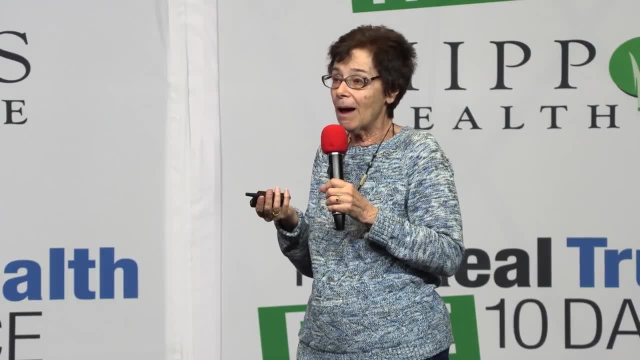 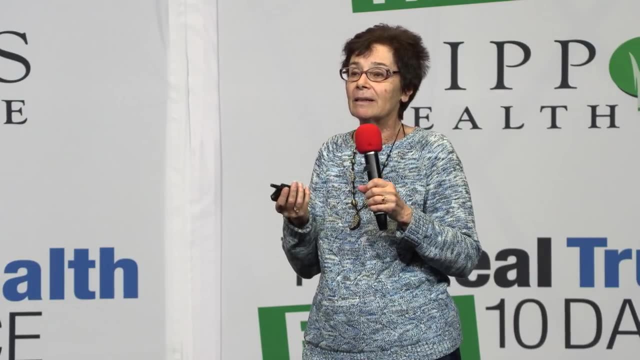 eating plastic. so this is apparently the plastic has some of the most important role in the life of the marine life, of marine life, some kind of odor attached to it that a lot of marine animals don't just eat it, because it's the only thing there. it attracts them to eat it. there was a 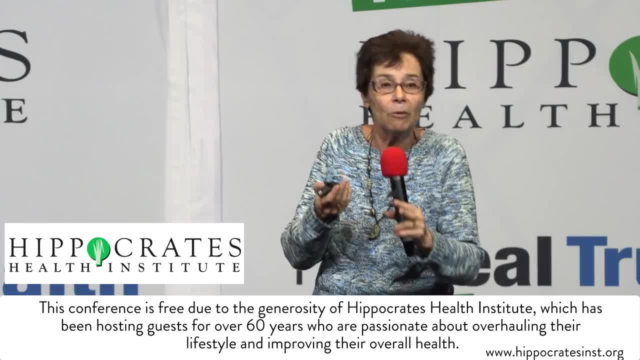 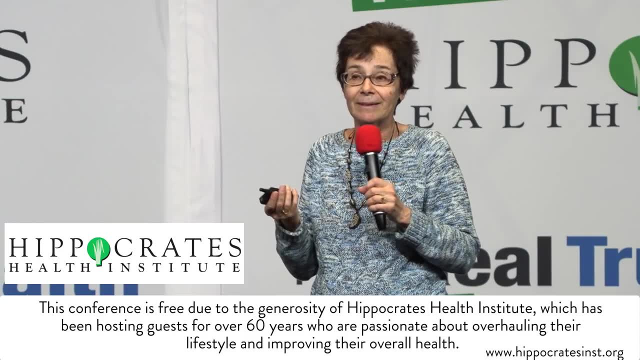 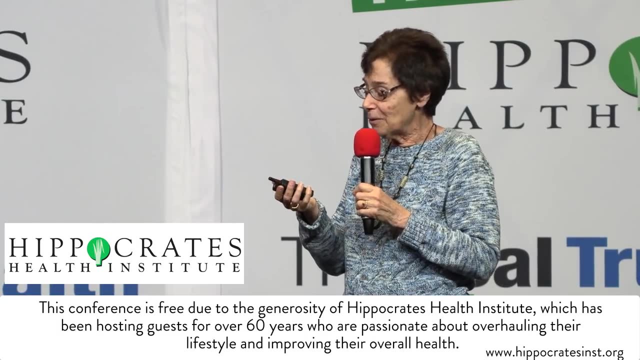 study done with some animals where they were offered real food and offered pieces of plastic, and they preferred to eat the plastic. so that's that's not adaptive behavior, but that's what they do. this is just an overall view of how much is going in and where it comes from. 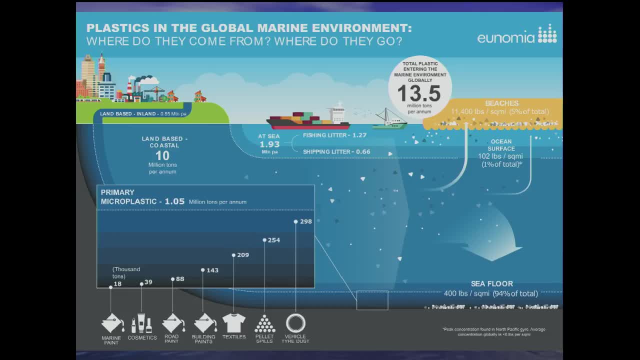 I guess the major take home message is that 10 out of the 13.5- whatever million, whatever it is- let me see million tons per year- 10 of those 13.5 are coming from land-based, so that that's where we have to look is on land for the where it's. 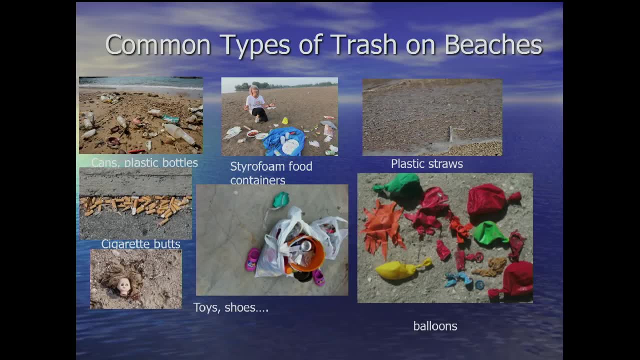 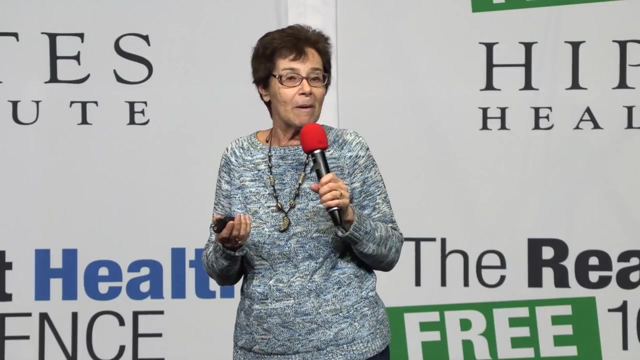 coming from. here's the common types of plastic: on beaches we find plastic plastic bottles. we find styrofoam straws, cigarette butts, toys, shoes, balloons- you've probably all seen this plastic bottles. i was offered one to have on my deus in case i was. 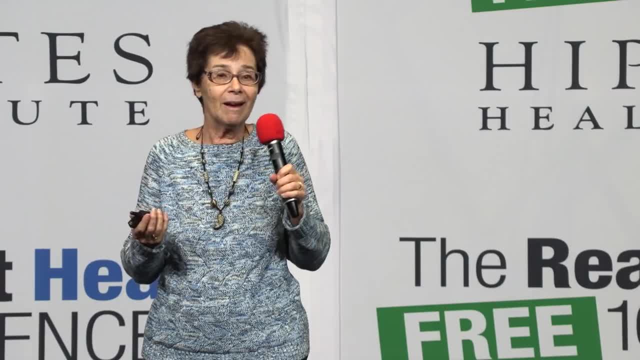 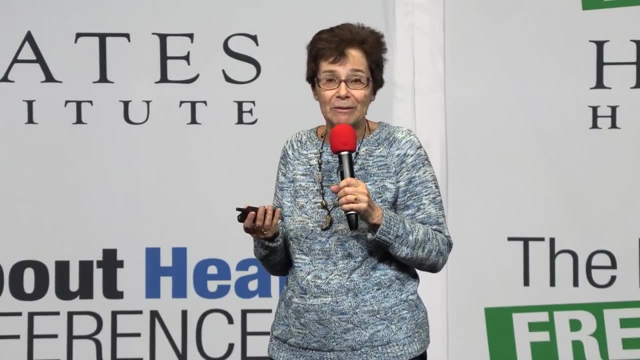 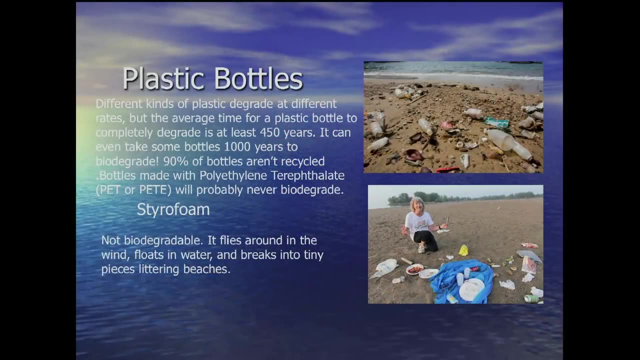 thirsty, but i turned it down because i didn't want to be having a plastic bottle. i tried to avoid plastic bottles. you should have a refillable bottle and fill it up and and not keep buying plastic bottles of water. bottles take forever to degrade- uh as as all plastic doesn't, and they're. 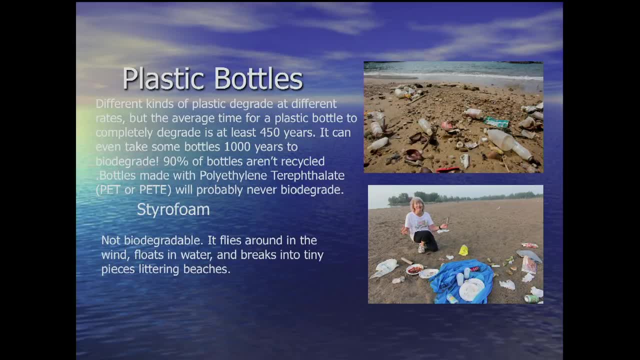 mostly not recycled. a lot of things that say they're recyclable doesn't guarantee that it actually is recycled and they don't degrade. styrofoam is one of the worst, because it breaks up the plastic bottle and it's not going to be recycled. and it's going to be recycled and it's. 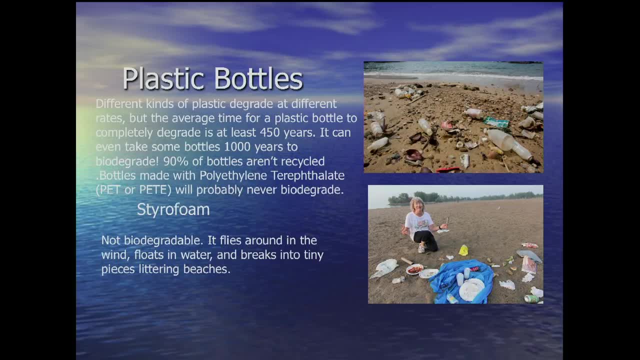 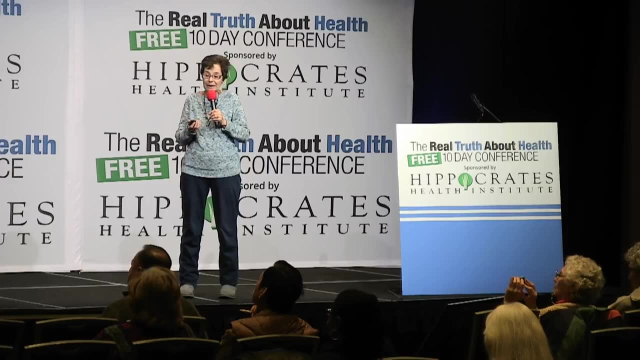 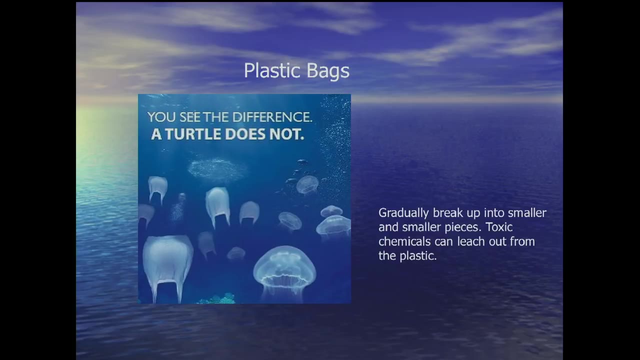 up very readily into small pieces and it blows in the wind and it floats in the water and it it litters the beaches and it blows all over the place plastic bags. so you see, uh, this is just showing you how a turtle might mistake a plastic bag for a- um, a jellyfish, and they eat them. 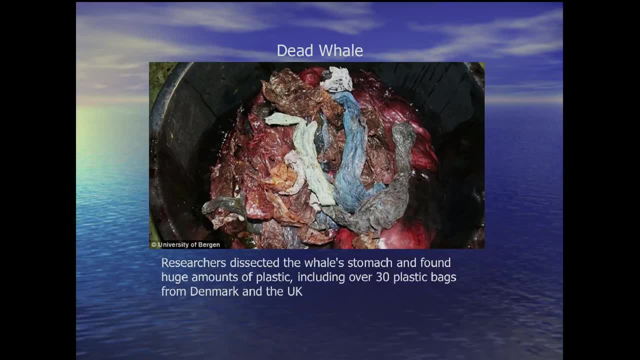 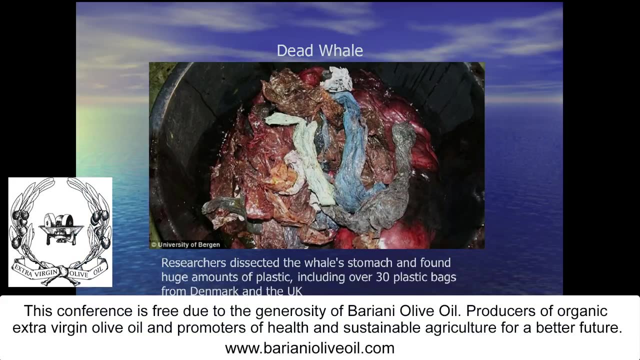 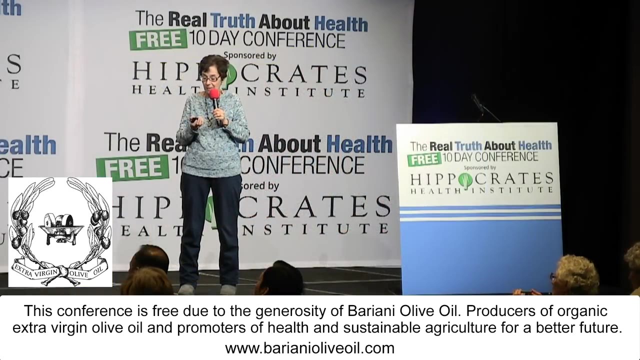 this is the inside of a dead whale whale washed up on a beach dead. they opened it up and this is what they found. they found huge amounts, including 30 over 30 huge plastic bags. this was in in europe and that's the insides of that whale's stomach. so again, like that dead bird, can we prove that the 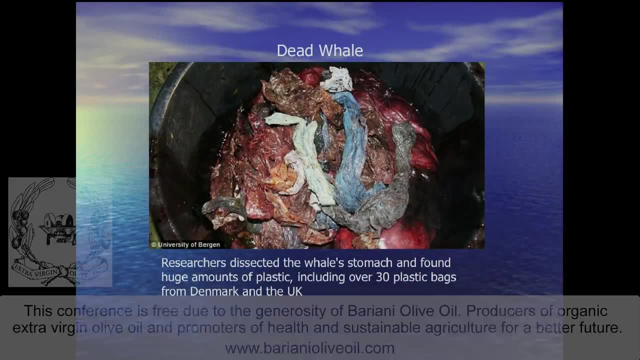 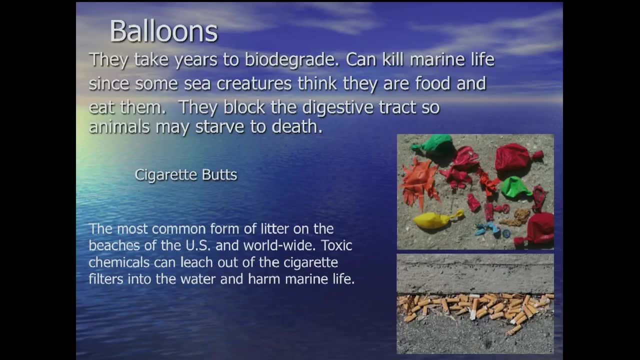 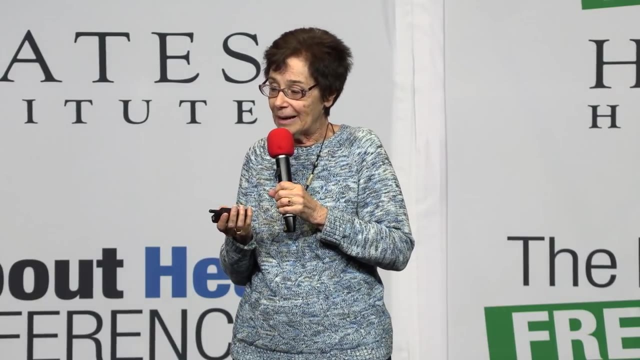 whale died from a stomach full of plastic. probably we can't prove it, but i think we all know it. balloons: we like to release balloons when there's a celebration. it may not be a very good idea. they take years to biodegrade and they kill marine life too. we find lots of balloons broken. 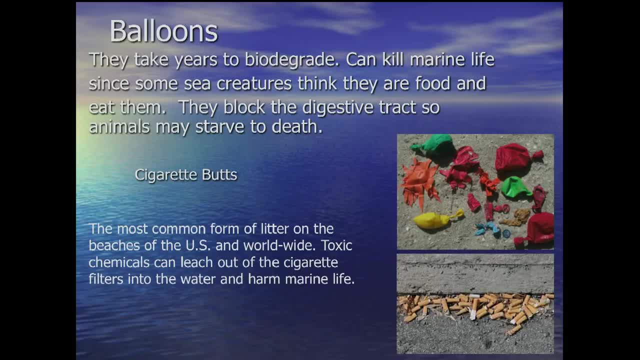 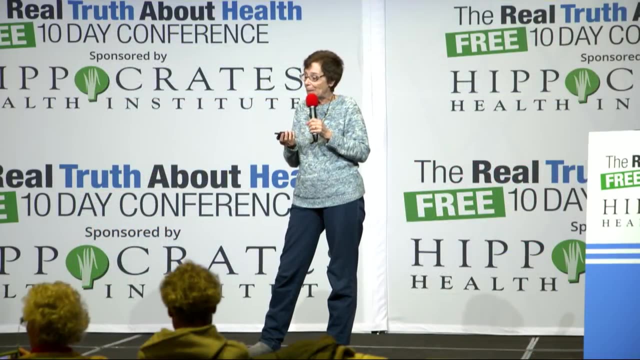 up, not intact, but broken up balloons in the digestive tract of marine life. and then there's cigarette butts, which is the most common, if you count individual items. uh, counting individual items of cigarette butt is a whole lot smaller than a plastic bottle. but the the filter material is. 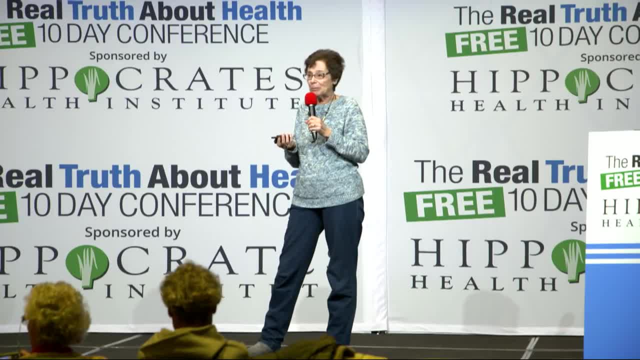 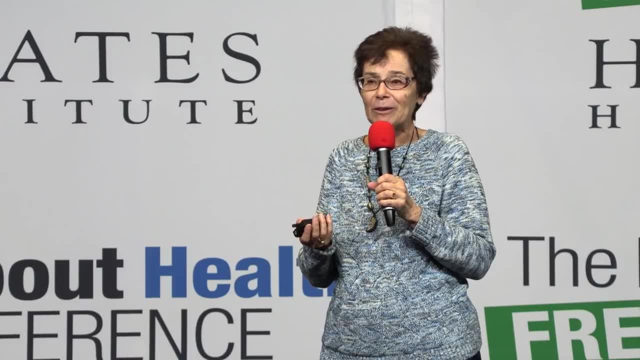 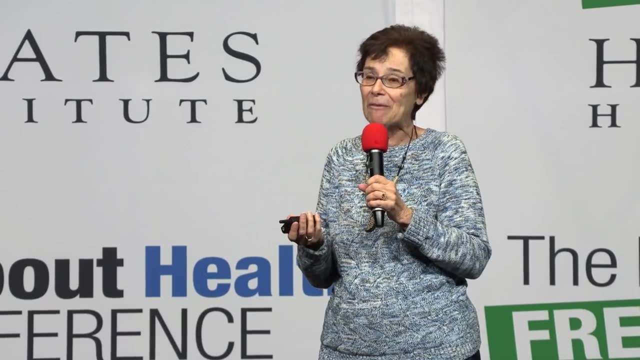 plastic. and it's not only plastic with the problems of plastic. it has all the nasty parts of tobacco stuck onto it. the filter is there to prevent the bad stuff, all the carcinogenic stuff in the tobacco from getting into your lungs. so now we have the filters with high amounts of toxic stuff on it. 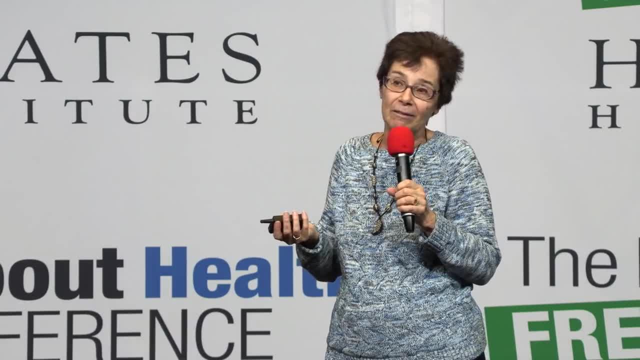 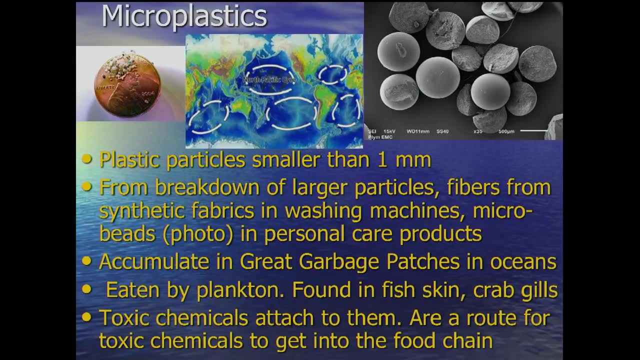 littering the beaches and getting eaten, of course, by marine animals. and then here's something that you may not have heard of: there is stuff called microplastics and they're. you know, you can see from this penny here the size: they're like a couple, a millimeter, a couple millimeters down to being microscopic. and, um, where do they come from? they? 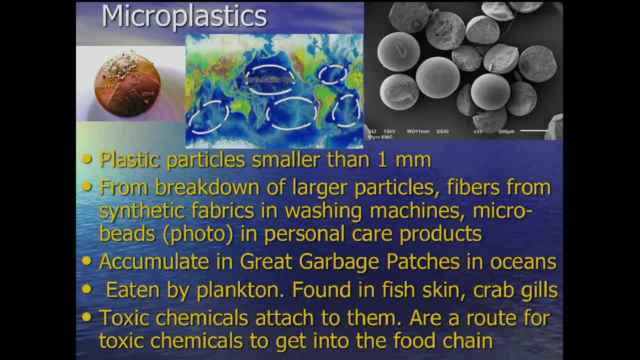 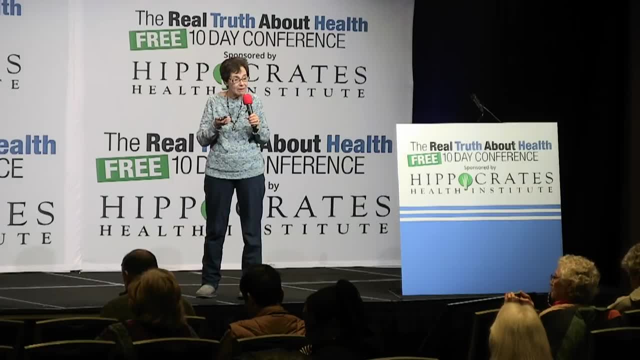 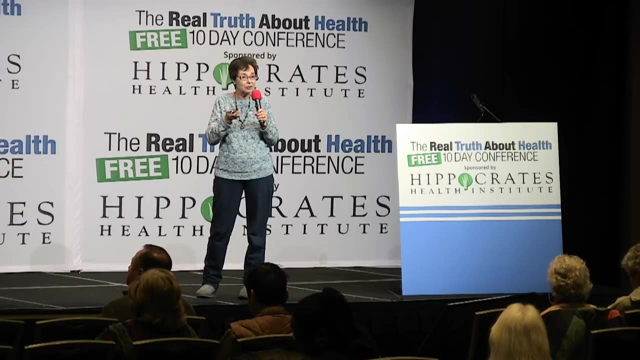 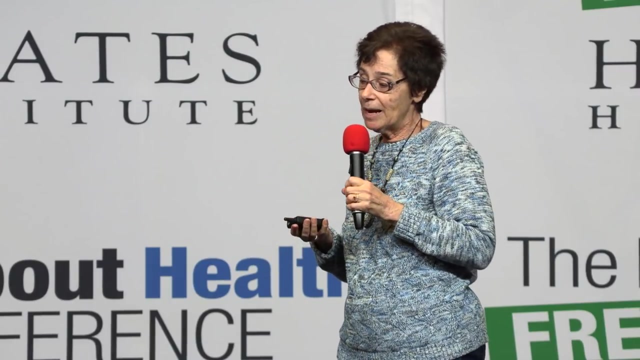 come from a number of sources. one is the breakdown of bigger things. secondly, is fibers from our clothing that we wash in washing machines? uh, clothing releases microfibers too small to get trapped in the washing machine, goes down through sewage treatment plants and into the water. 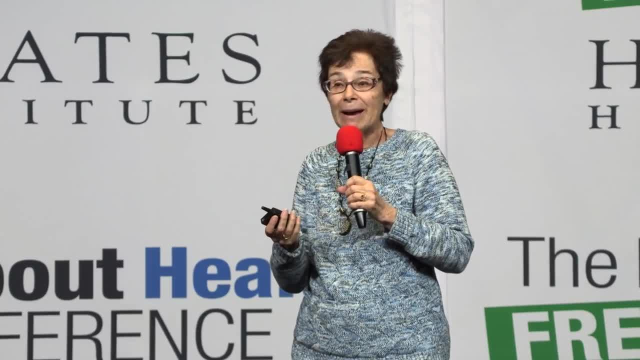 and sees. micro plastics are micro plastics that are shaped like this, microplastics magically on tap, and these plastics allow us to rise too, and if this wasn't going to be an accident, then it wouldn't be a there must have been. do you know? there's going to be overflow, or if we just didn't evolve with? 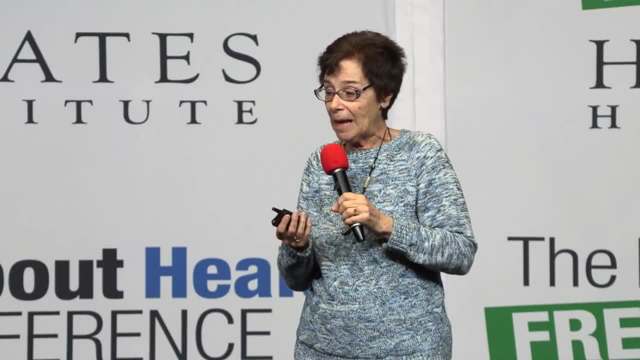 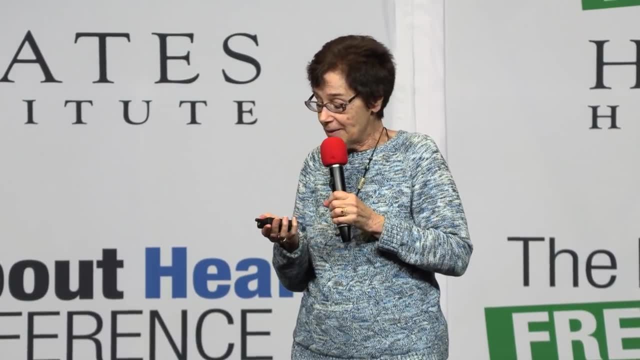 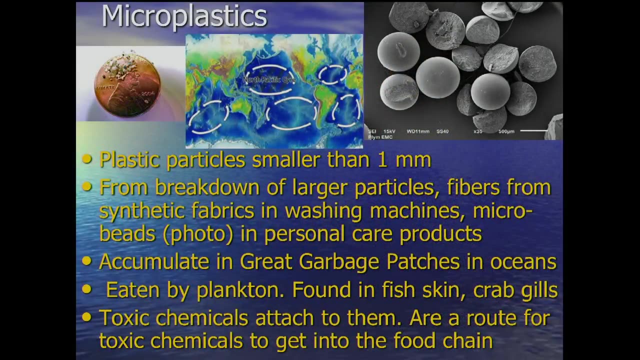 things like that- a fiber long, skinny thing is- are the most abundant type of micro plastics that we find. and then there's this kind. that's a sphere that wouldn't come off clothing. that wouldn't be a breakdown. that was purposely. those were called micro beads and they used to be put into personal care products like skin you. 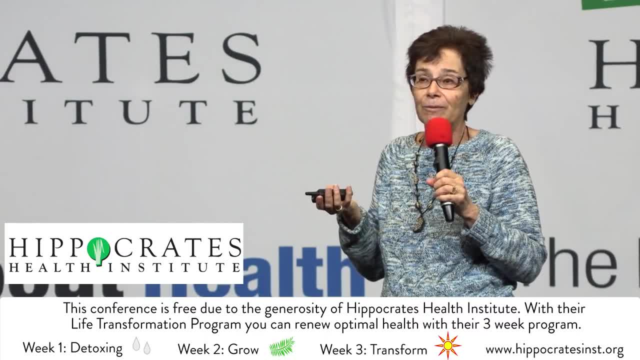 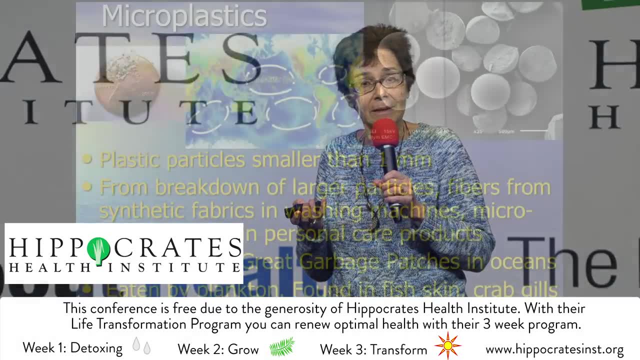 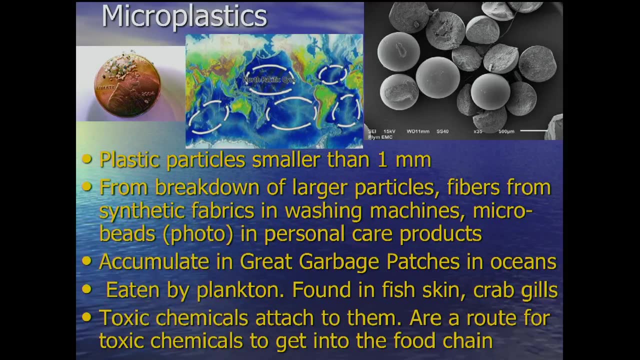 know abrasive things for freshening your skin, getting rid of the dead skin and stuff like that. these were banned in the US a couple years ago and so they're no longer on the market here. they're probably still on the market some other places these small pieces of plastic will accumulate. in the major there's one. 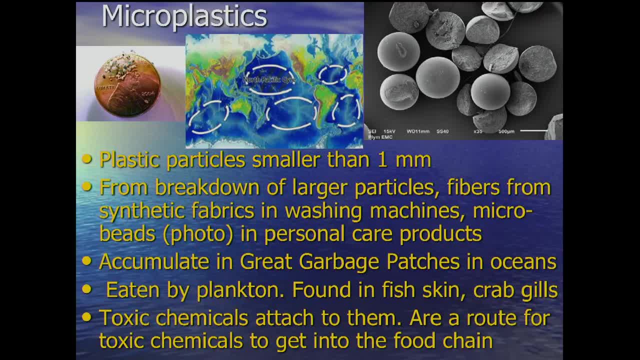 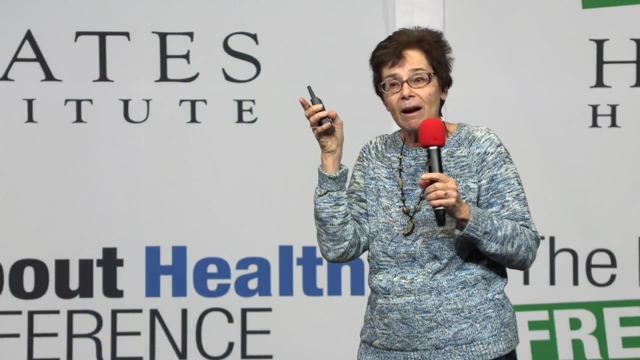 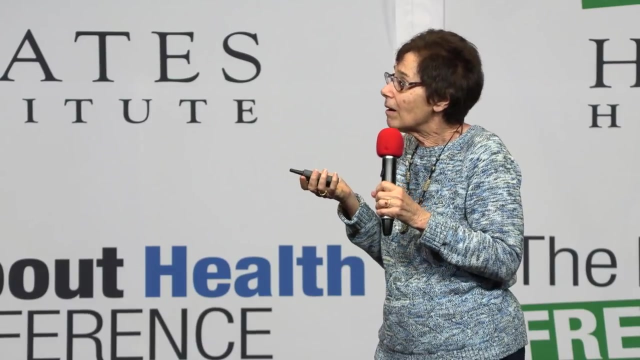 called the great pacific garbage patch. you may have heard of that. there are these patches, these areas, in all the major oceans. each ocean has circular currents going around and in the center, where the currents aren't, is where all this floating litter accumulates. so you find a greater density of plastic and other litter in. 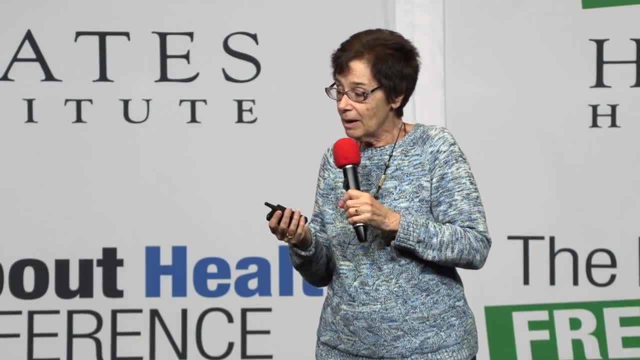 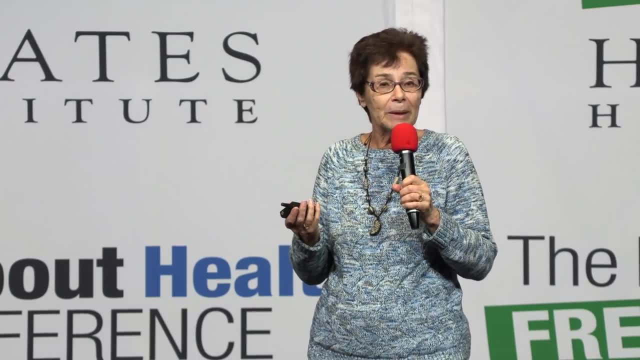 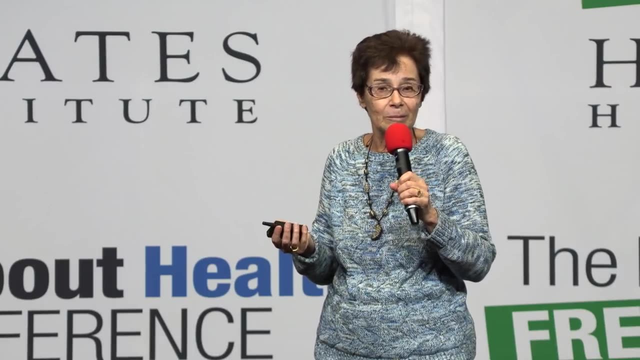 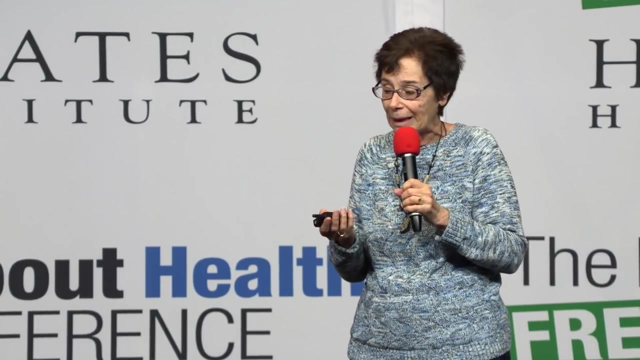 those areas. so another problem with the plastic is that they, just like the big pieces, the little pieces get eaten by little animals. the big, the big, bother balloons and whatever- get eaten by bigger animals. the micro plastics get eaten by tiny animals: baby fish, little plankton and so forth. and to make matters worse, like I, 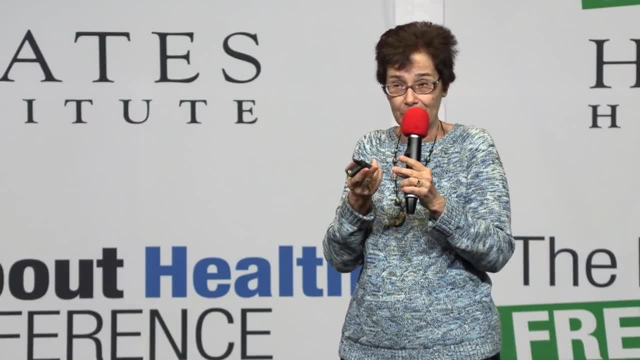 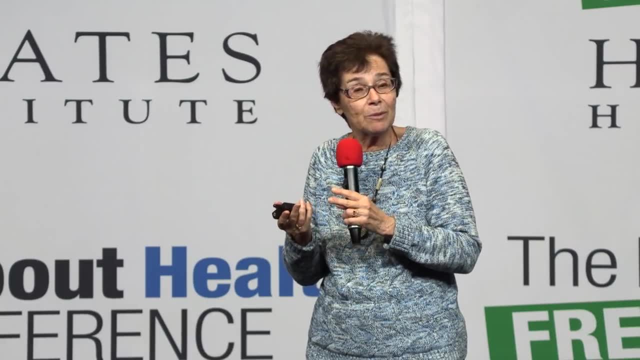 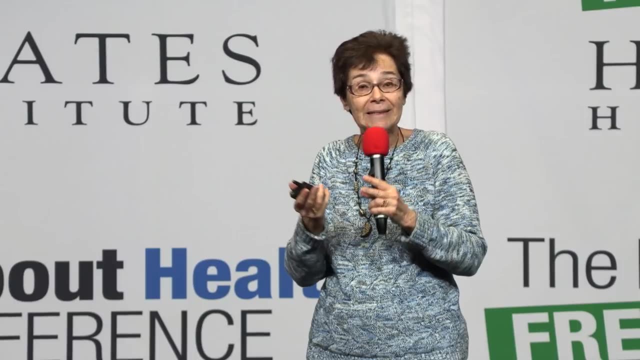 had mentioned for the corals that the term my back disease-causing Bacteria attached to them at, which is a problem for carls. chemicals- toxic chemicals that may be in the environment also will attach to the micro plastics so that, as the fish or the plankton eat them, they 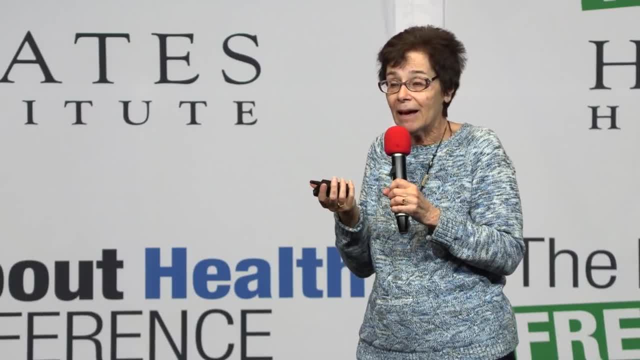 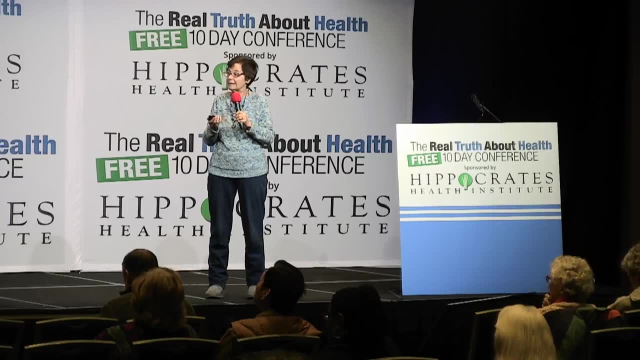 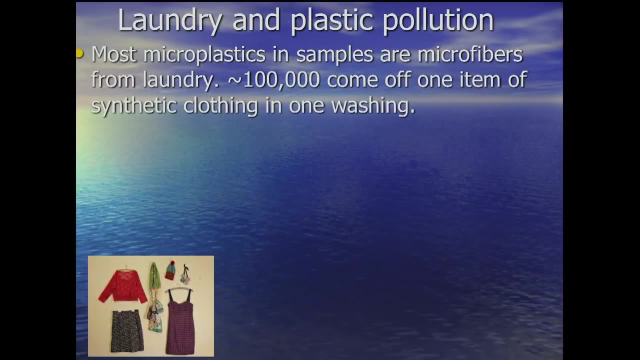 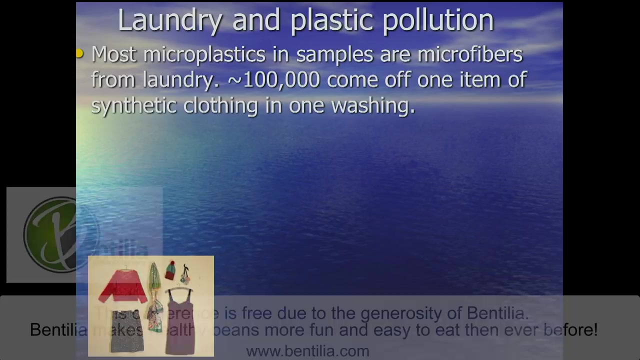 are getting not only the plastic itself but some toxic chemicals as well. so this is a way for toxic chemicals to get into the food chain. all right, a little bit about your clothing, your synthetic clothing. most of the micro plastics we find our micro fibers and they're coming again from our synthetic clothing. and 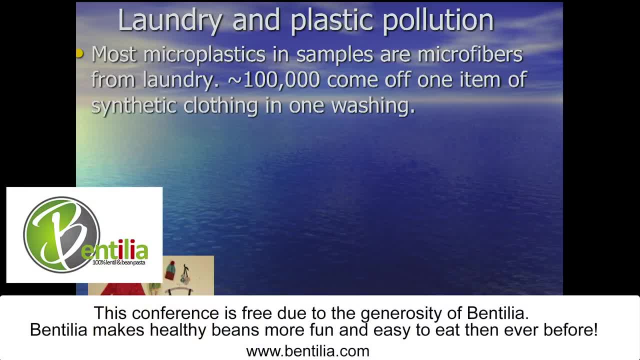 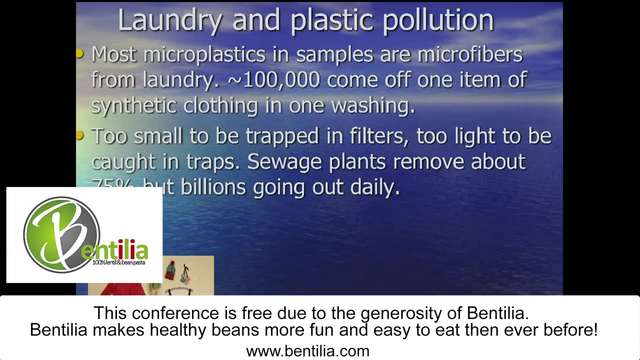 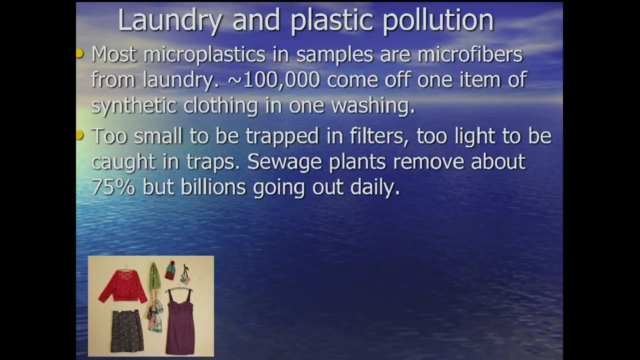 one item of clothing can release a hundred thousand of these tiny fibers in one washing and again they don't get trapped in the washing machine. sewage plants release perhaps three-quarters of them. I mean remove. sorry, sewage plants remove about three-quarters of them, but that still has many billions going out. 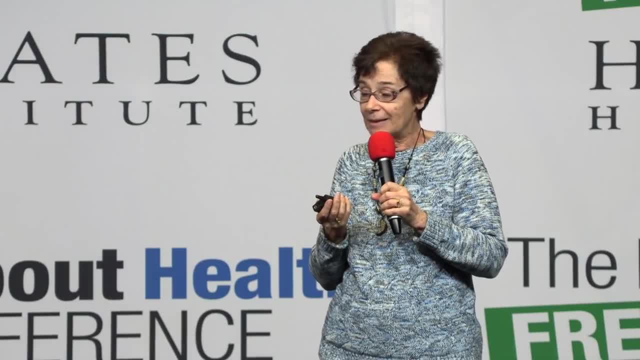 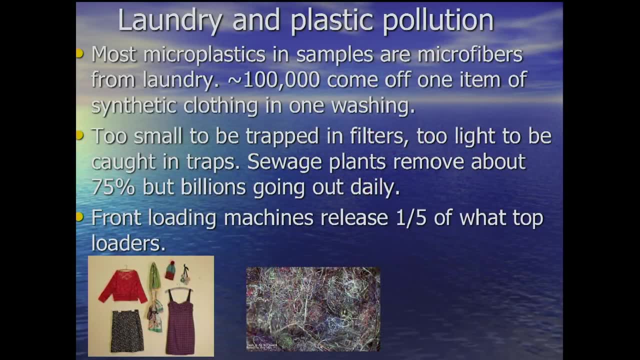 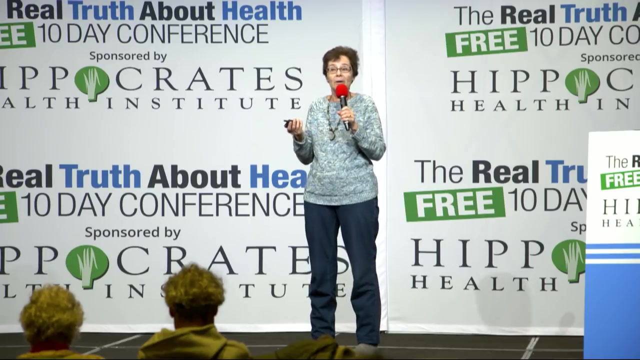 into the waters every day, and this is just a microscopic look at tangle of microfibers. an interesting thing that was found was that front-loading washing machines release much less than top loaders. so if you have a need for a new washing machine and you're thinking of buying one and you want to do the right thing by the 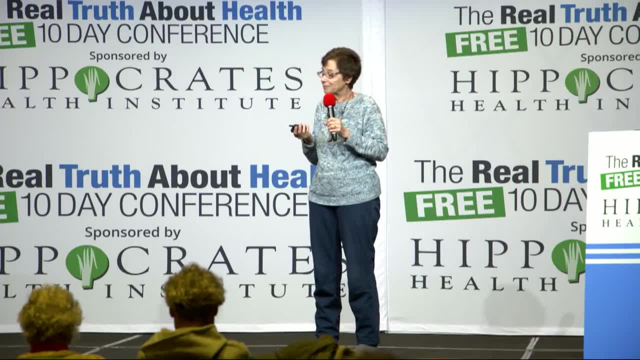 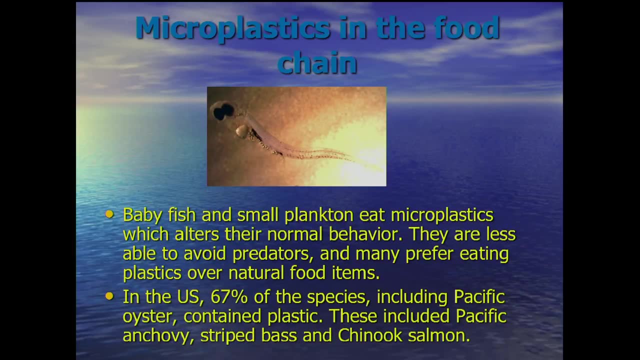 environment. a front loader would be better. ok, just looking at this picture of baby fish and small plankton: eat the microfiber plastics. I think you can see along here little spheres. this is an experiment in the, in the laboratory, and, and I said before, they seem to prefer eating. 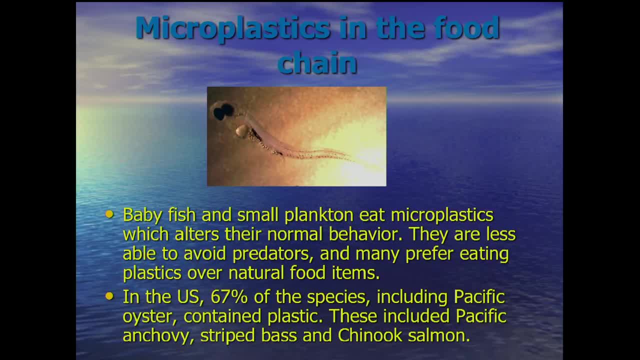 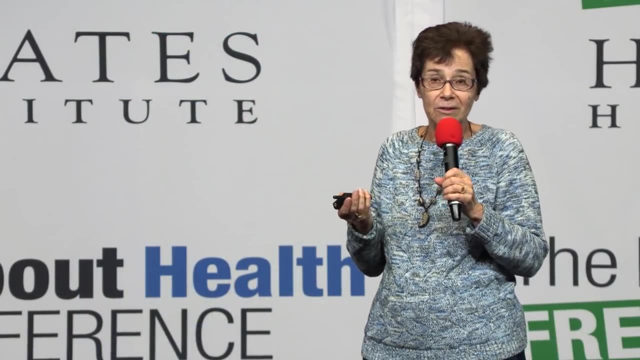 plastics to other things, and most species that have been looked at have found been found to contain plastic, including the commercial fish species. we, and, of course, the shellfish, so we are. if we eat fish or shellfish, we undoubtedly have microfibers in in us as 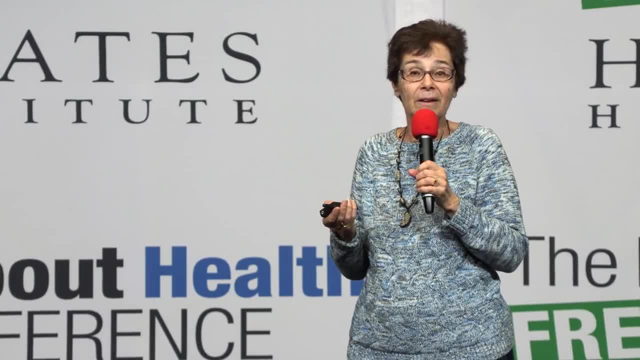 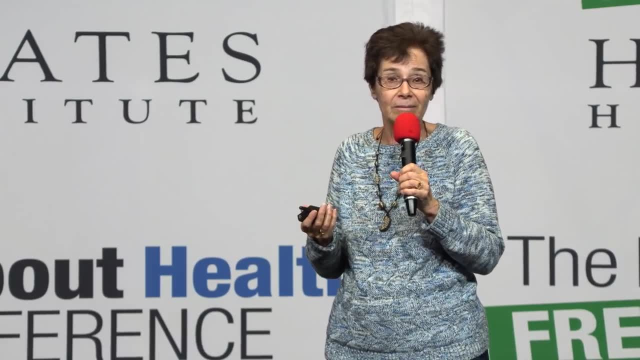 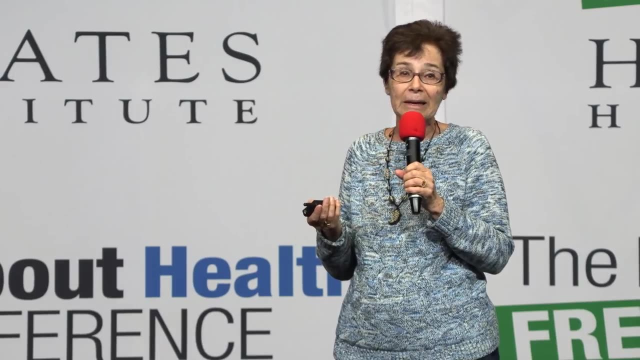 well, micro plastics anyway. and other thing, talking about health, food and all, a lot of people think sea salt is healthier than regular salt sea salt. of course, if you evaporate the ocean water and have the salt behind, all those plastics are in the salt. so on your head. 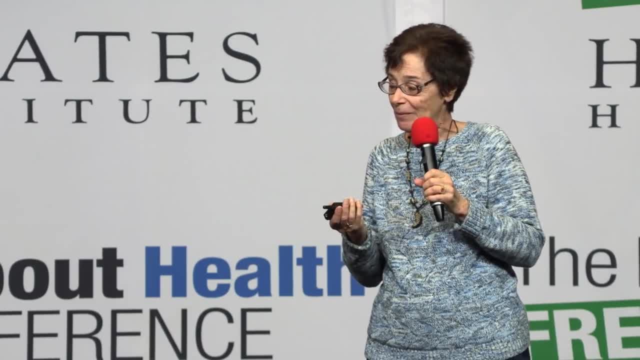 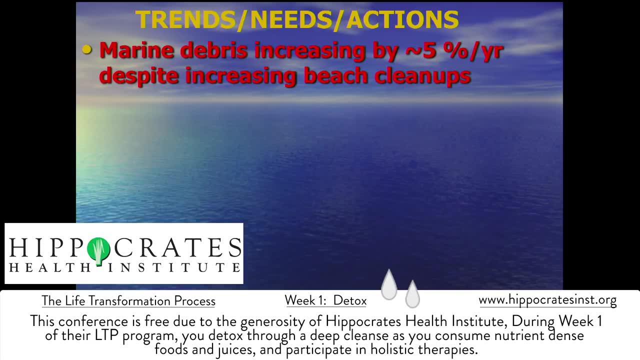 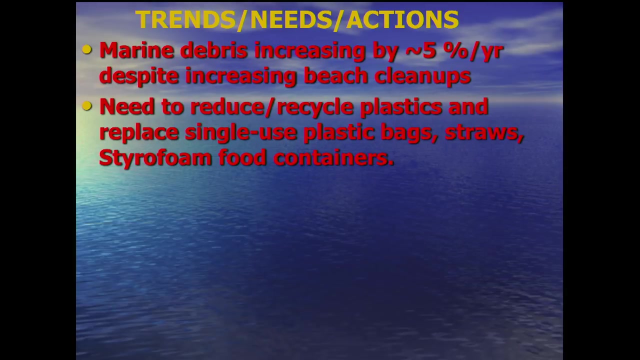 healthy sea salt is giving you more microfibers. ok, summarizing what's going on with marine debris: it's increasing each year, despite more cleanups. we need to reduce and recycle plastics and replace single-use plastic bags. and hooray for Suffolk County. Suffolk County did it with plastic bag, you will know. 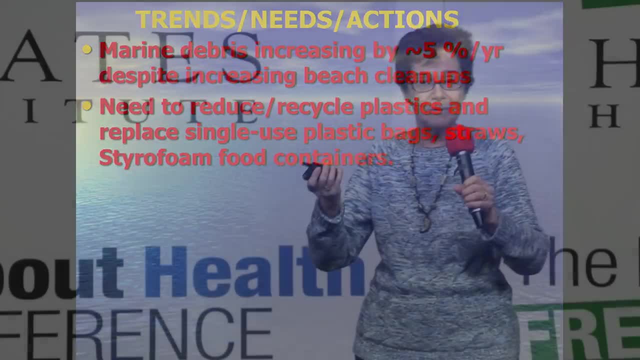 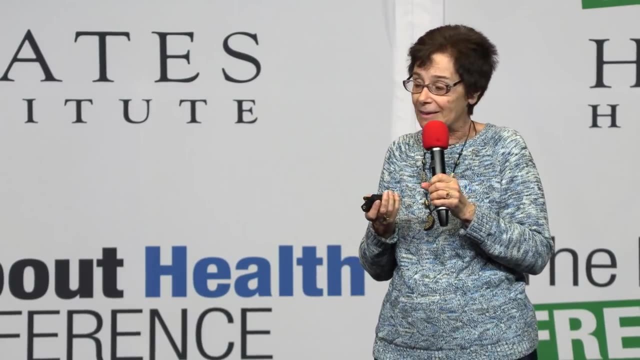 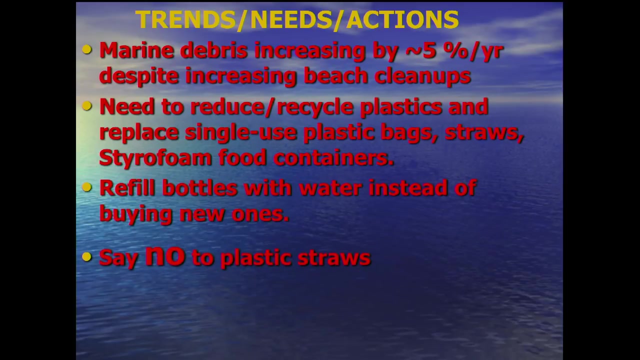 that I was hoping to hear a cheer from you all. anyway, we need to do something about styrofoam as well. you need to refill bottles and not continue buying new plastic bottles for water and say no to plastic straws. how many have you been to? 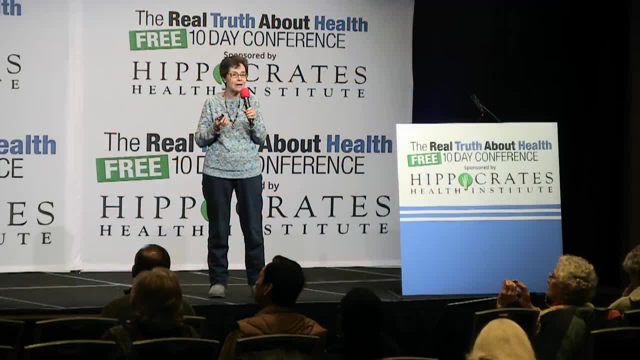 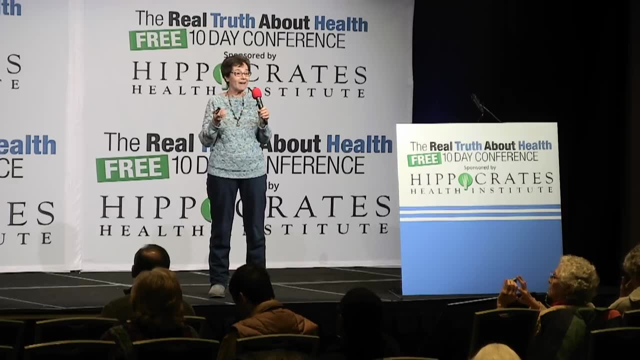 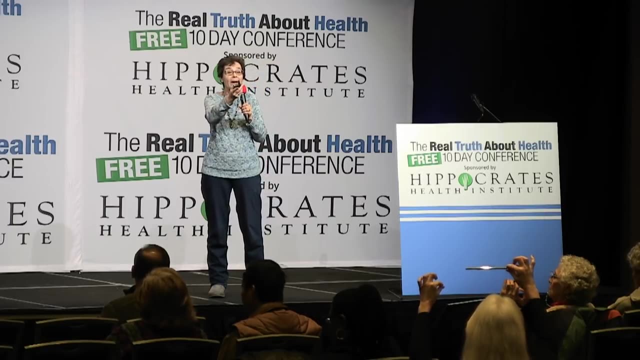 a restaurant. you order a cold drink and it comes with a straw in it, and you never asked for it, but the straw is there sitting in the drink. if they would only have a policy of giving straws out only to people who requested it, or you have your own straw, but if you don't happen to have your own straw, try to. 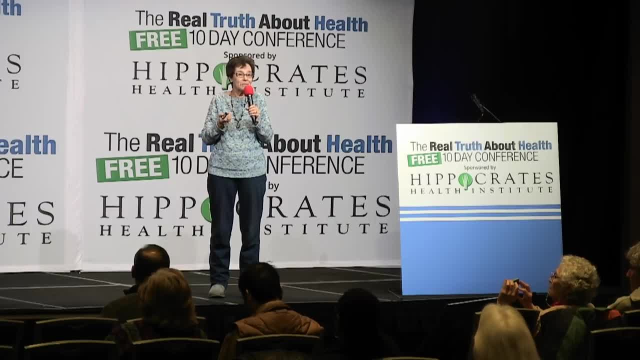 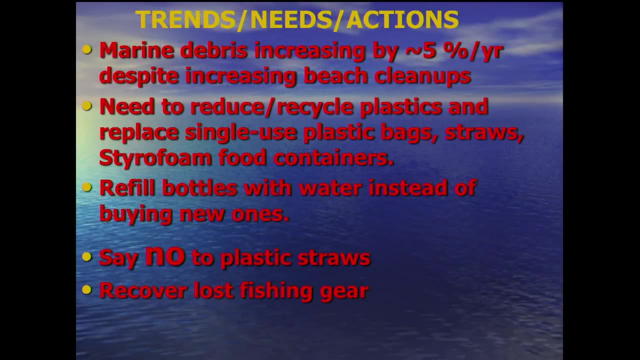 remember, when you order it, to tell the, the, the wait person: no straw please, because that will come even if you don't ask for it. and recovering lost fishing gear- lost fishing gear is a- is a big problem and that's not a matter of carelessness and not thinking. this is this stuff that is valuable to the. 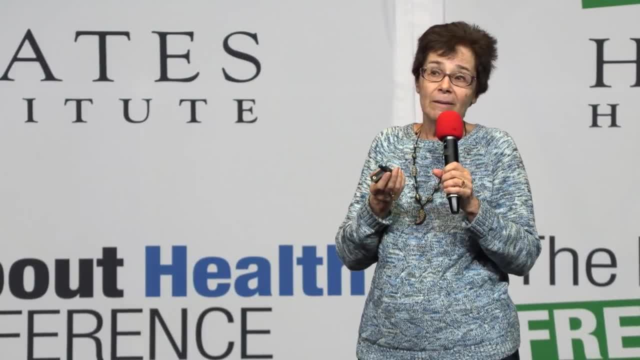 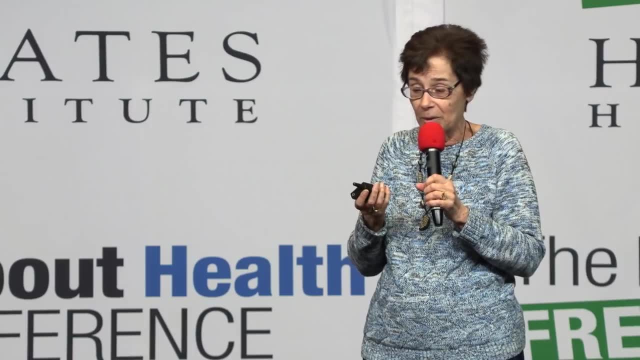 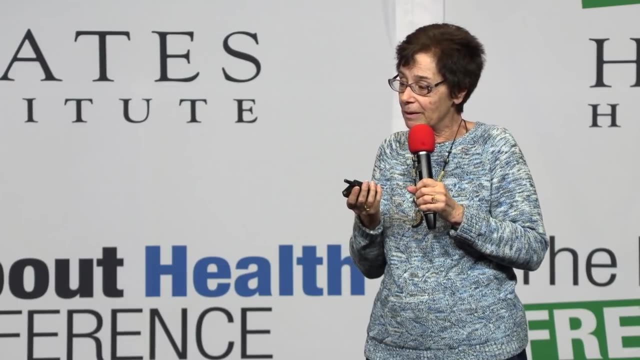 fishermen and it got torn away in a storm or something. this is not a matter of the fishermen's negligence. it's a bad news for the fishermen as well as for the environment. okay, some more. here we have federal legislation phasing out micro beads we have, you know, these are the 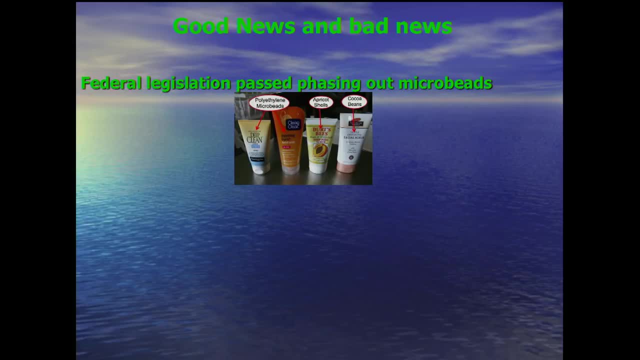 personal care products, some of them that had styrofoam and then it's not styrofoam, the plastic beads and then some others that are using natural thing. there's plenty of stuff that can be used to abrade your skin. many countries and counties and towns have had bans or fees on plastic bags. many places are.